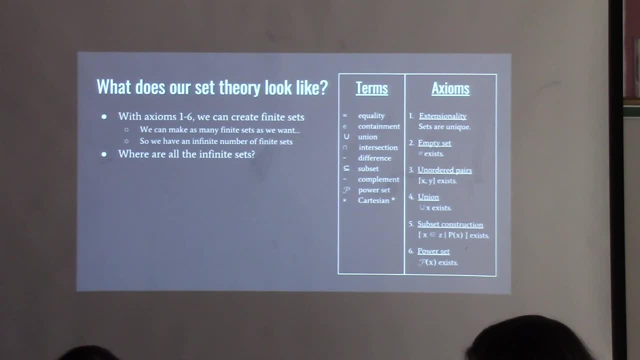 So we can only make finite sets with these axioms. In particular, we can make an infinite number of sets, each of which is finite. Someone agree? That seems totally clear. Okay, so we need more axioms, because we also need infinite sets. 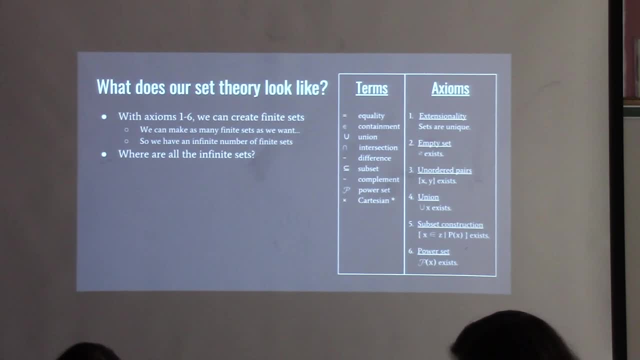 If you are the kind of people who are following Zermelo-Frankel's axioms, you are trying to reconstruct the full power of like Cantorian mathematics, Just without the paradoxes. So you want all the goodies like ordinals and stuff like that, right. 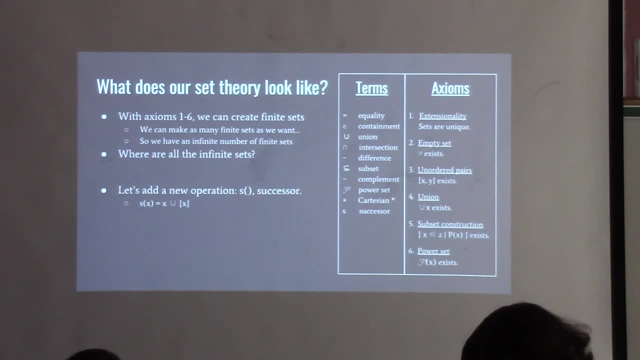 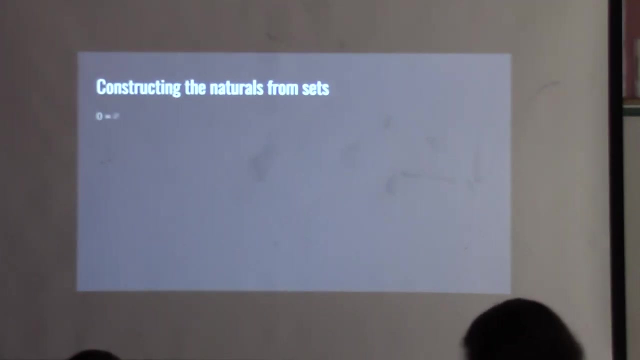 And if you're going to make ordinals, you need some infinity. So let's define a new operation, the successor operation, which has its old definition of successor. The successor of a number is just x, union that number. And now we can see how we can construct the naturals slash, you know ordinals, using the axioms of set theory. 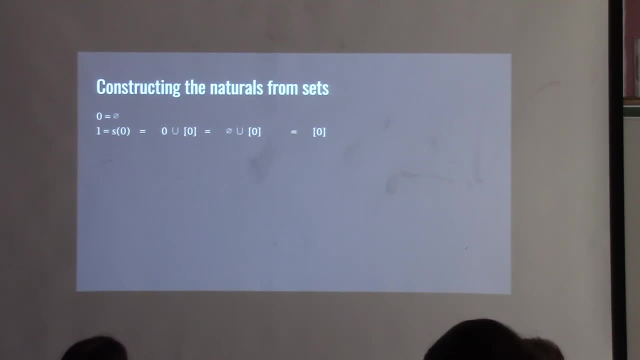 We've seen so far, Zero is just the empty set. One is just the successor of zero, which is zero. union second-taining zero, which is the set which is the empty set. union the second-taining zero. So it's just the second-taining zero. 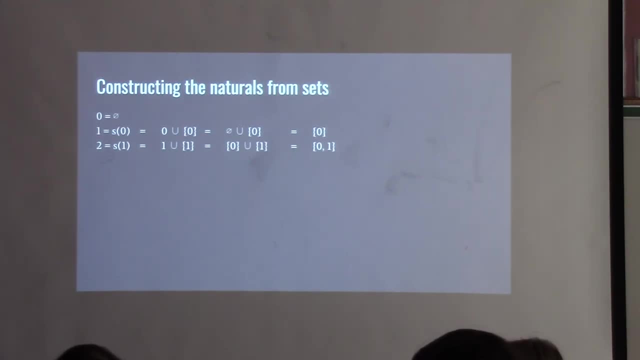 And then et cetera, et cetera. This is like review right Two is just the successor of one, so it's one union, And all of these operations that I'm performing are operations that I have the power to perform via the ZFC axis. 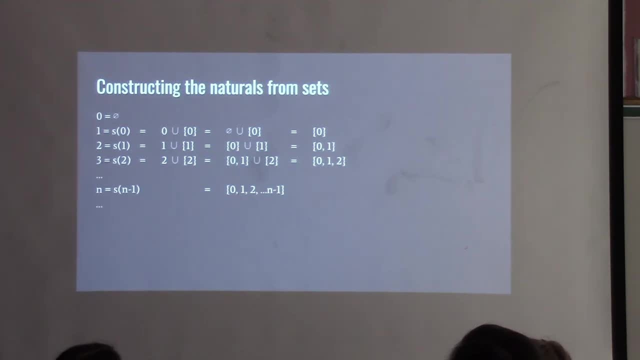 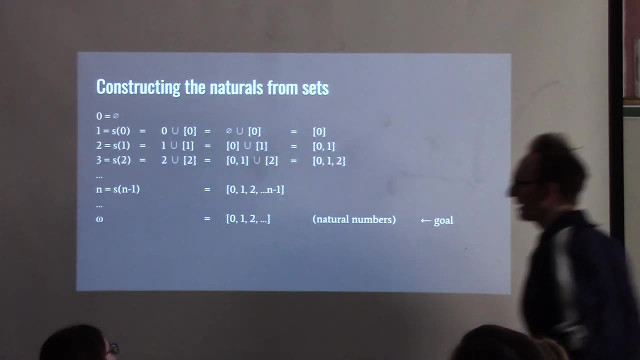 And we get a boom-boom, and this goes on and on forever And, in general, n is just the successor of n minus one. Okay, So I don't need omega. I like, want omega, And I have no ability to construct the set omega yet. 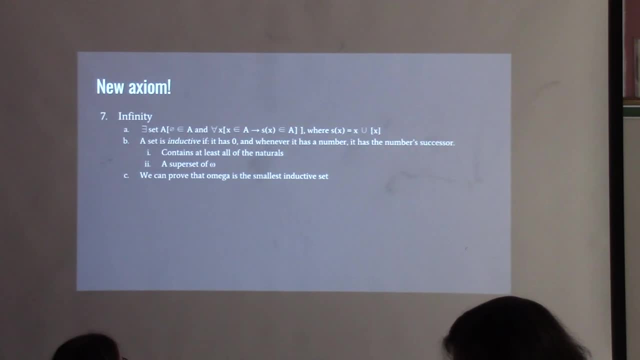 So I need to be able to make the set omega. Okay, Skipping over a lot of the details, we have a new axiom. This new axiom is called the axiom of infinity And, loosely speaking, it says well, okay, let's read it. 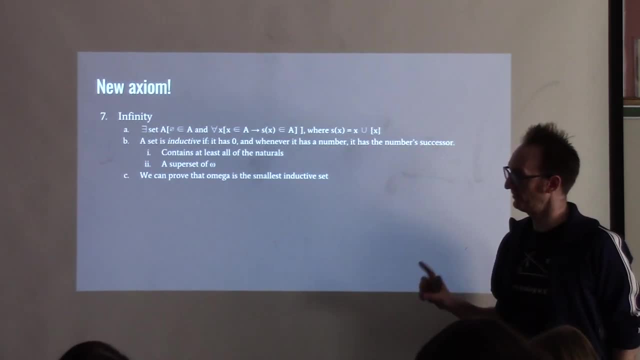 It says: okay, define a set as inductive if it has zero and whenever it has a number in it, it has the numbers successor. Okay. So, intuitively, an inductive set, the natural- would be an example of an inductive set, because they have zero and whenever they have a number, they have the next one. 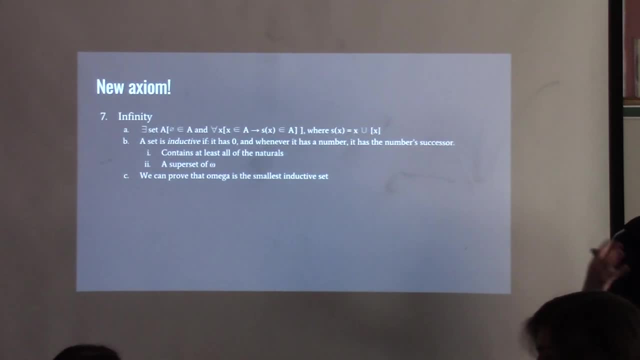 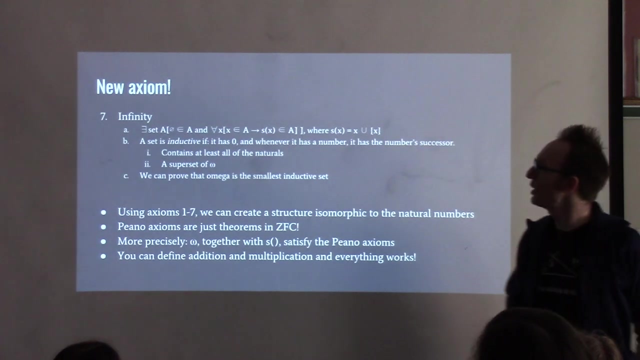 But also the naturals, like plus, like some monsters, would also be an inductive set, right? So essentially, an inductive set is any set which, when it has a number, it has that number successor And then a very high-level proof ensues, which I'm skipping, in which one 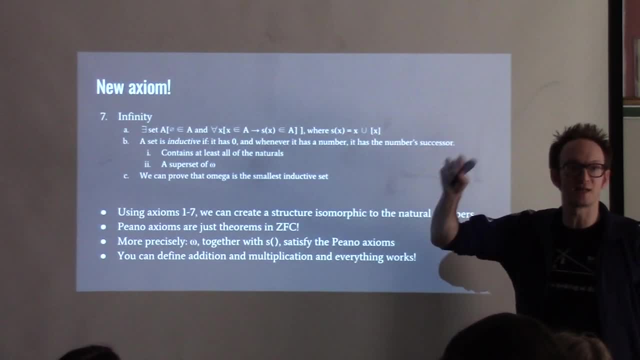 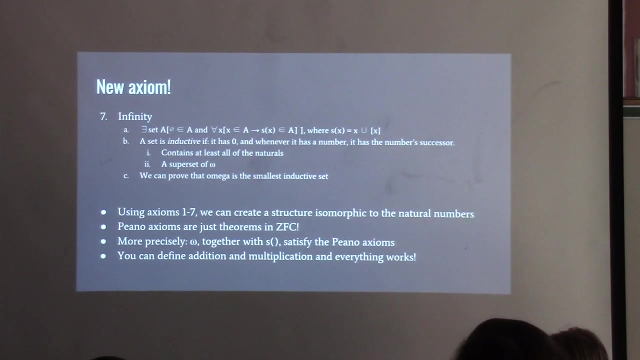 One proves that there is a smallest inductive set and one defines that inductive set to be omega. Or one defines omega to be that smallest inductive set, You sort of. There's like a minimal set which is inductive, And what the axiom of infinity does specifically is it asserts the existence of a set which both has the empty set in it and, whenever it has something in it, it has the successor in it. 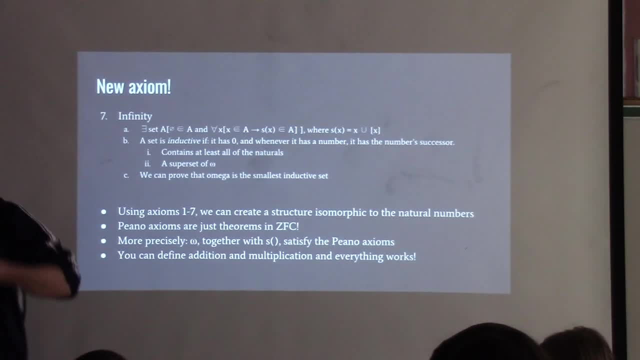 Okay, Get it. So I have this. I sort of give myself this ability to create these infinite sets And then I, Using axioms so far, we could show that there is a least one. That least one is omega. Okay, 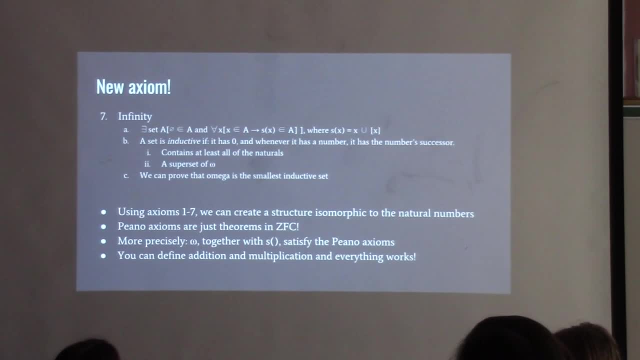 This is pretty much where. So okay, So using these axioms, we can essentially construct the entire natural numbers. This is the von Neumann construction. Yes, Are we sure we won't get a loop like s of 1 is 2, s of 2 is 1?? 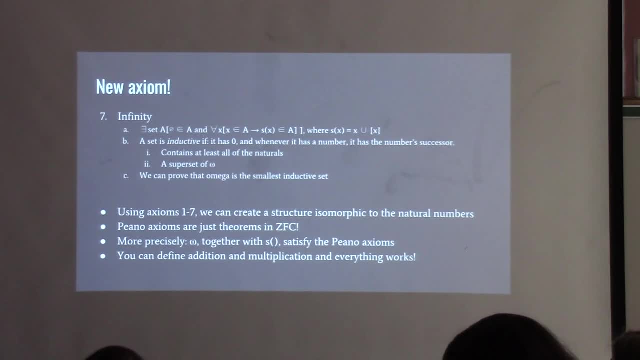 Yeah, I think we are pretty sure because, based on the definition of successor, I think that just can't be right. Yeah, Like, how do we prove our sets don't loop? I guess, Wait, but stop. It's not saying for any successor. 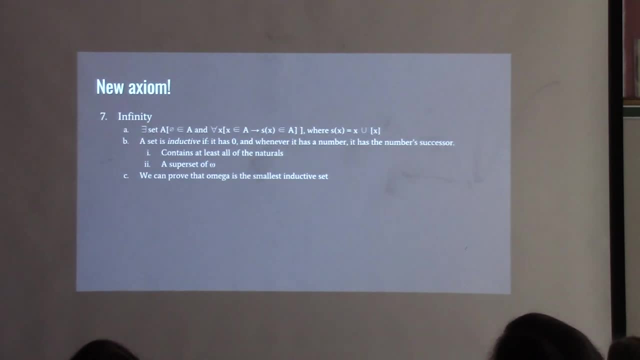 It's not a model, It's that successor, That specific. Yeah, I'm specifically defining the successor operation as a set operation And that certainly, Yeah, Okay, So we now have like Suddenly, like we kind of did it right. 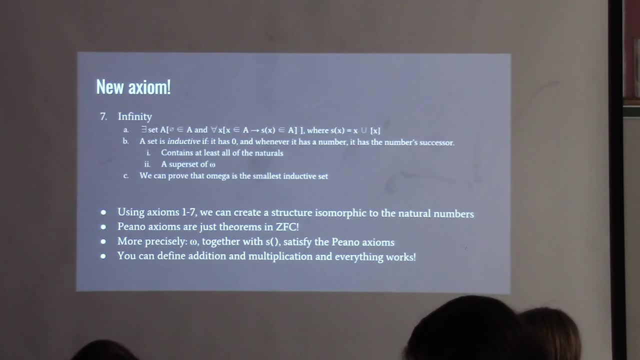 The goal was for set theory to be strong enough to be able to have all, To be able to represent all the axioms of piano arithmetic. and we just have. So you can prove every one of the piano axioms. you can prove holds in ZFC. 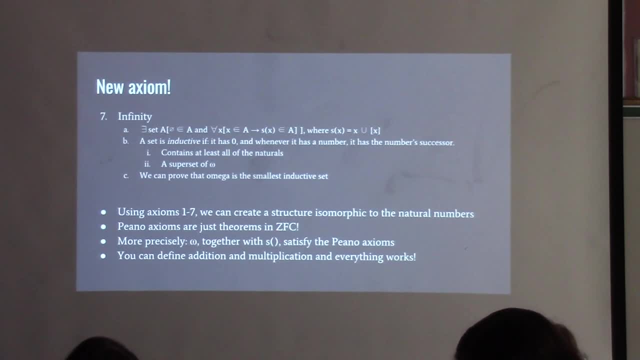 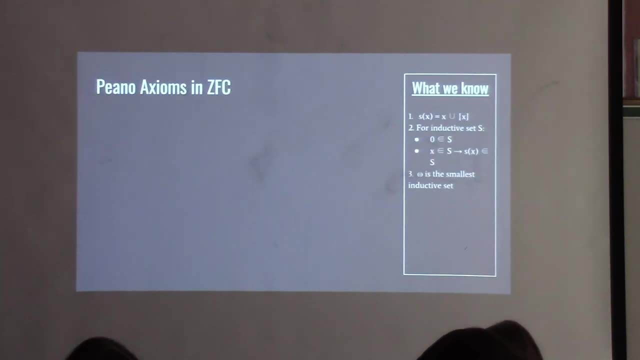 It all just kind of works out. In other words, if these set theory axioms like do what they're supposed to do, then I have proven sort of piano arithmetic from these set theory axioms. And what are the set theory axioms? 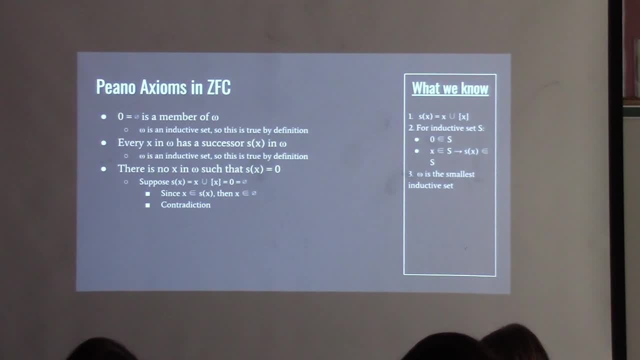 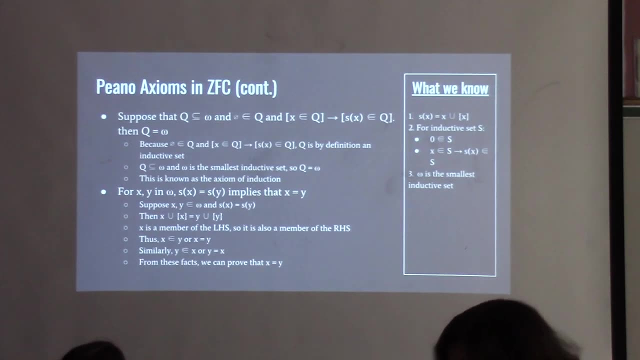 What are the piano axioms? Well, that there's a number zero? Okay, of course there is, because we have an axiom that says it, And then every number has an accessory. It all just works out All right. Blah, blah, blah, blah, blah. 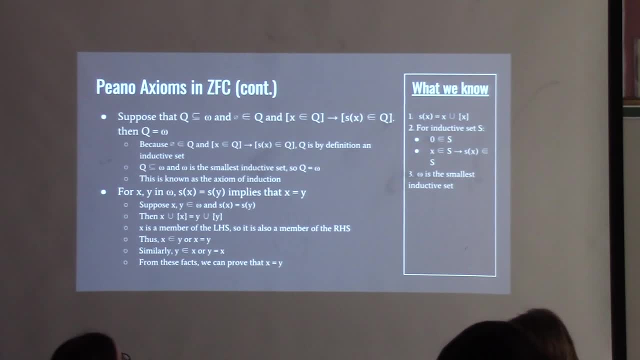 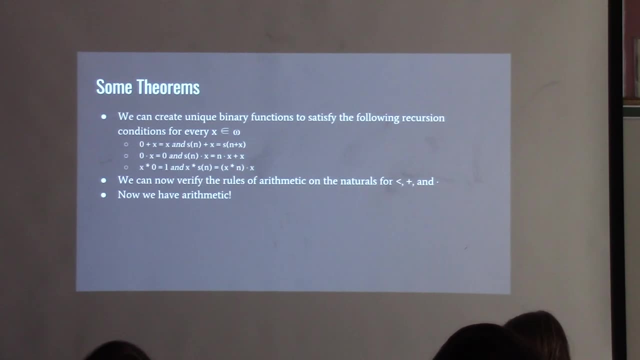 Oh, this is the proof. No, we're not doing it right now. This is the proof that, Basically, this is the proof of induction from our definition of omega. Check it out later. It all works out. You can construct addition. 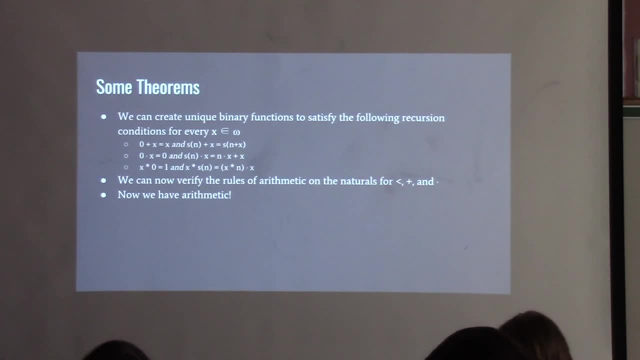 You can construct multiplication And now every sort of arithmetic operation is really just a set Theoretic operation And you can just verify that all the rules of arithmetic work And they're all just theorems that can be proven, All right. 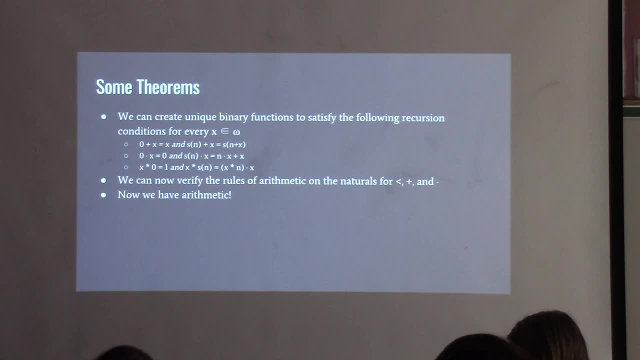 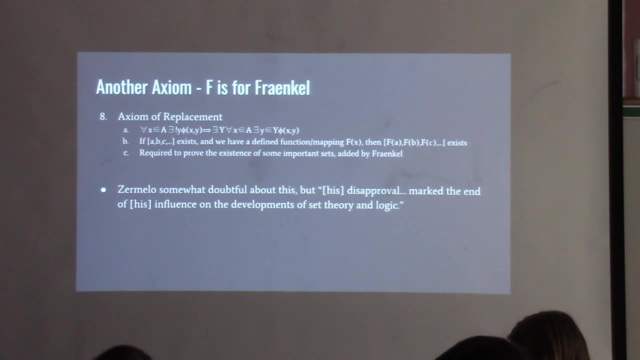 This is like kind of where Zermelo stops, although this is even sort of better. We gave the cleaned up version of everything that Zermelo did. It's later on, when Frankel. I said this on Friday. Frankel rephrases all the axioms in first order. logic clarifies what a first order, what a predicate is. 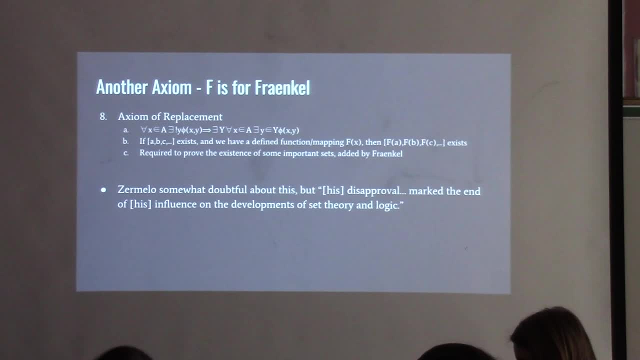 He also finds that there are some things, Things that you might want, that you can't do in Zermelo's original axioms, And so Frankel adds in some very difficult to understand axioms which we're going to skip through kind of quickly, such as the axiom of replacement. 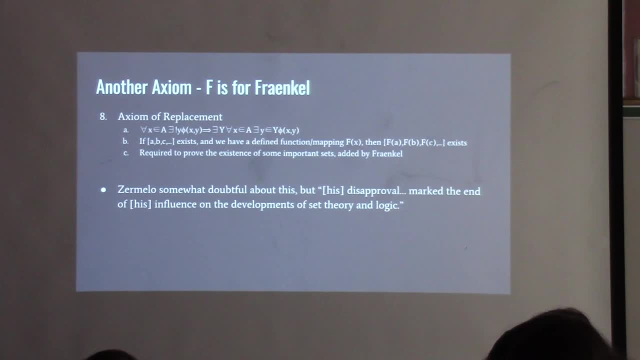 The axiom of replacement. I've spent hours of my life trying to understand this axiom. It's really hard And it's basically very, very roughly speaking. It, roughly speaking, says that if you can define a function and if you have a set, then you have the set of images of that function. 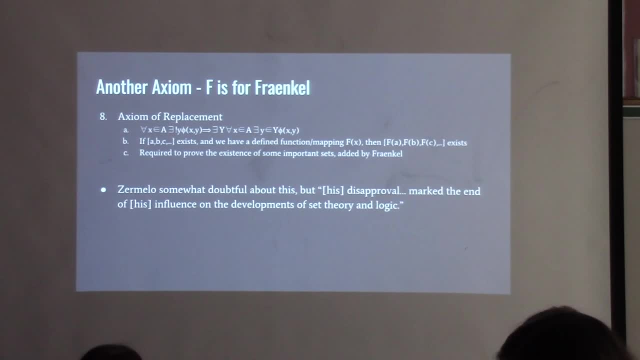 But the details are more complicated And there are some obscure sets not of interest to the average mathematician but of interest to some people who are interested in them, of some advanced sets which require the axiom of foundation to prove, For example. 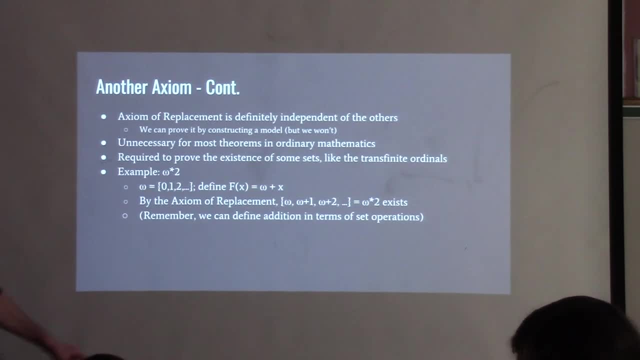 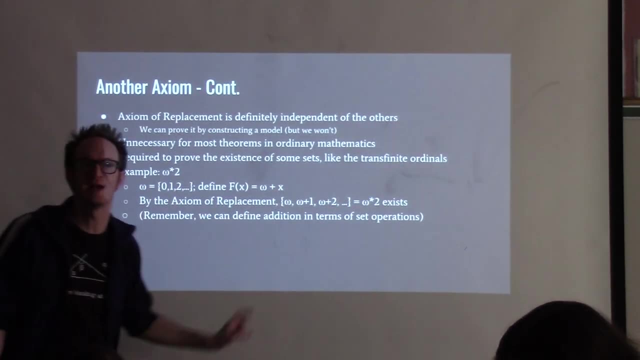 For example, if you want the set- this is a typo, I fixed it, but then I left my flash drive open, so this is the Google version. Let's just say- you know this happens every day- that you want the set omega, omega plus one, omega plus two, et cetera. It's not actually omega times two, It's just its own weird thing. I personally have never had a need for that set. But let's say you want that set. It can be shown that you cannot construct that set using the previous axioms. 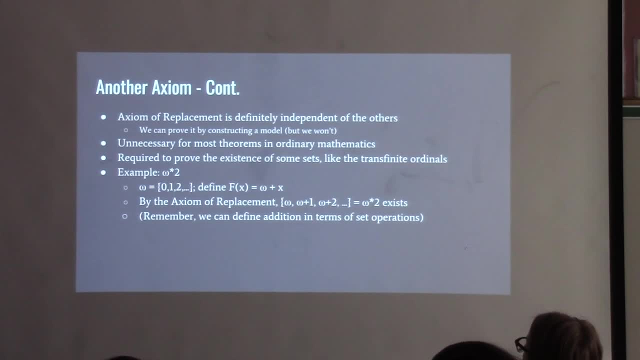 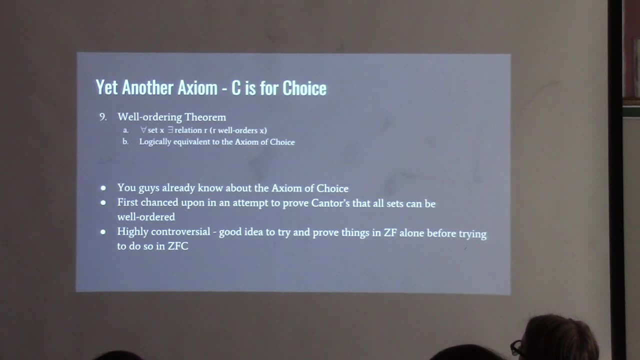 But with the axiom of foundation, With the axiom of replacement, you can OK. Then there is another axiom, which is the axiom of choice, which you now know about What's wrong. This is the bad axiom. This is the axiom that some people don't like and some people love it. 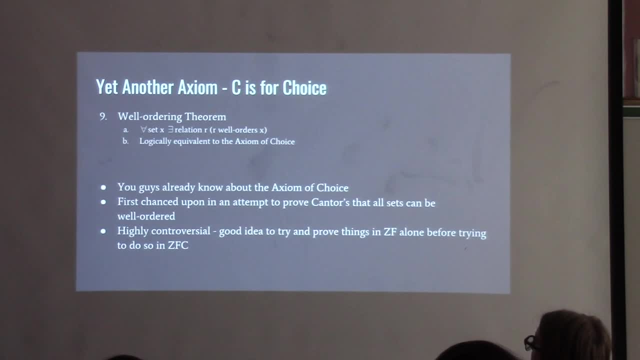 So the axiom of choice came up over the weekend presentation. But most mainstream mathematicians are in support of the axiom of choice, And so I think I said this last class, but maybe you didn't understand what I was talking about. The reason why it's called ZFC is because it stands for Zermelo-Fraenkel with choice. 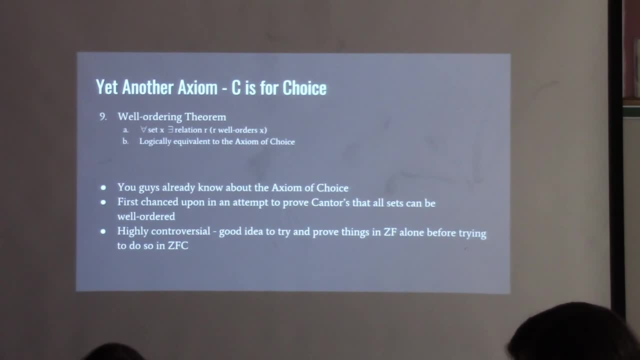 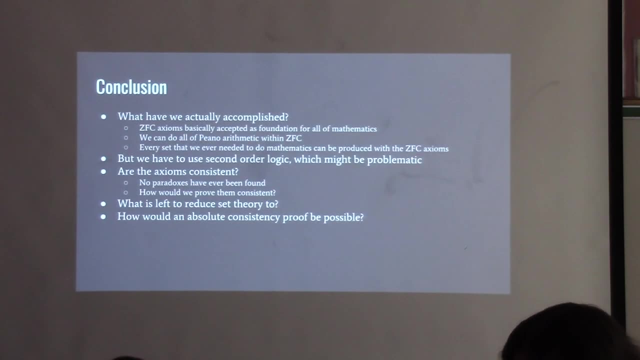 So when people say ZFC, they're explicitly including the axiom of choice in their axiomization. If you don't like the axiom of choice, then you take it out and you use just ZF. All right, So good. This is a good place to stop. 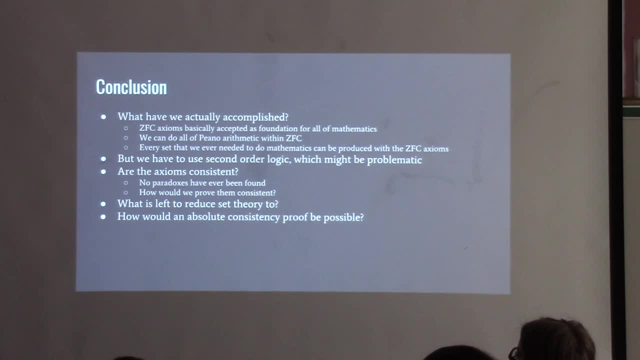 We could have gone into a lot more technical detail on various points And I even skipped an entire axiom, the axiom of foundation. So I'm really glad I skipped it because it's really weird, But basically OK. So this axiomization of set theory, it basically works. 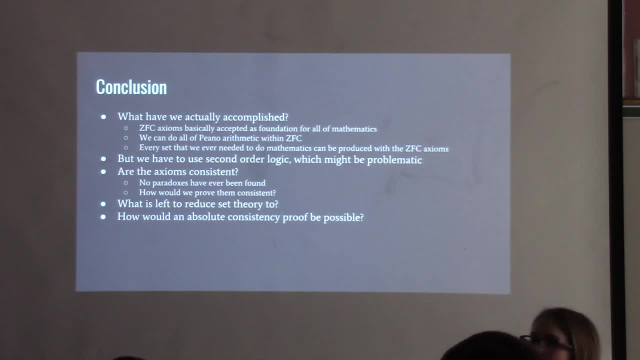 And what I mean by works? what I mean is every intuitive set, theoretic operation, construction, argument, etc. that had been used into the 19th century has now been formalized, And the precise power that sets are allowed to have has been sort of explicitly mentioned and delineated. 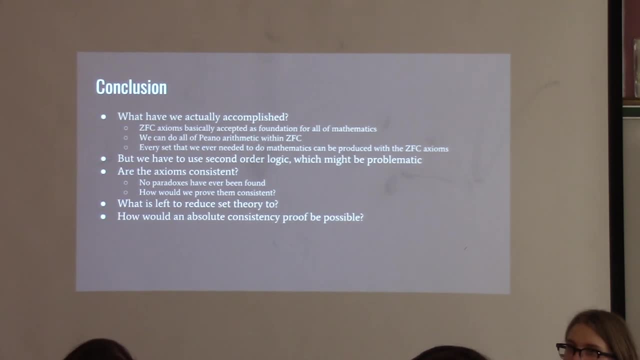 So, in other words, we axiomatize this branch of mathematics. Secondly, we have given our axioms enough power that they can do all the things that we need set theory to do. Set theory serves as a foundational role in mathematics, even up to now, even in 2019.. 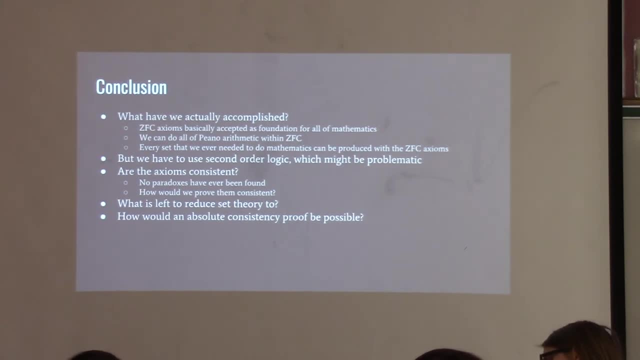 In principle, all mathematical theories can be stated in terms of just set theory. It's really down to the level of just ZFC. All mathematical arguments are really just long Fitch-style proofs in ZFC with many, many, many defined constructs. 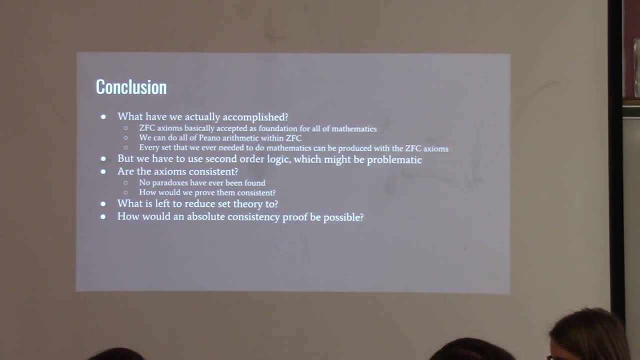 This is at least one interpretation with some current mathematicians. Can you get more information with ZFC, though You? when you get more information, you mean like the numbers actually are sets versus like something else. Right, like three is an element of four is not a set of numbers. 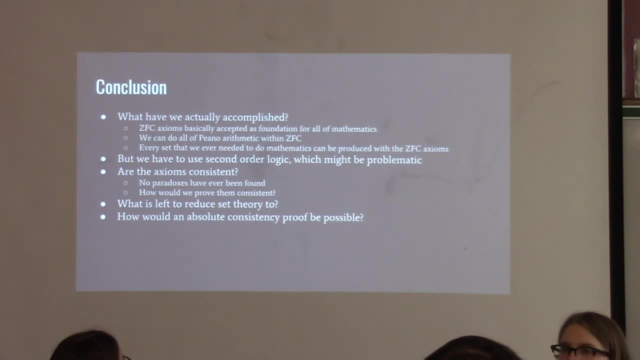 Yes, yes, He doesn't like. Eli doesn't like that When you're just doing arithmetic like three plus four equals seven, That's like a fact that you want. So check. Good. But what he doesn't like is that if you represent three as a set and you represent four as a set, 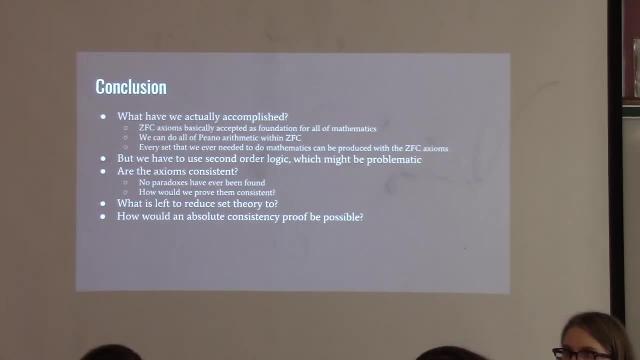 you represent addition as a function, which is a set, then he has a philosophical objection. You still get a theorem that is, when interpreted correctly, says three plus four equals seven. But he thinks that that's like too much or something, because really three plus four equals seven shouldn't be about set theory. 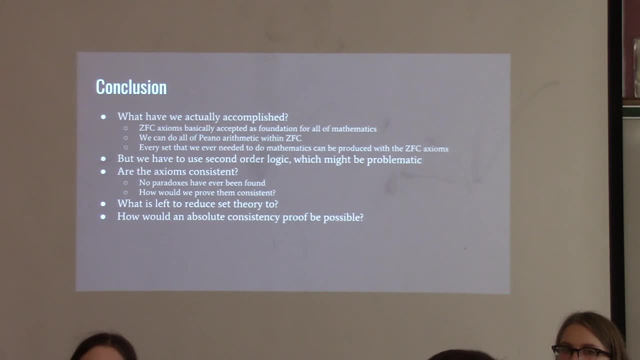 It should just be about numbers. Set theory should just be a model. He thinks set theory should just be a model of arithmetic. That's a slightly different position. OK, But at least every statement of mathematics can be written in the language of set theory at least. 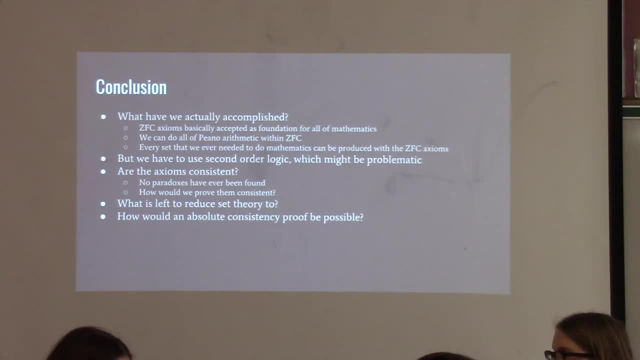 OK, The other part of what we were trying to do was we were trying to avoid paradoxes. So have we? We have to prove, We have to prove that Maybe we have. It feels like we have, It feels like we avoided the paradoxes. 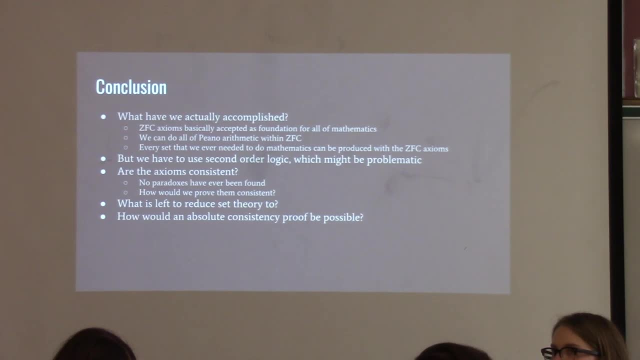 Or at least we avoided the one paradox that we were aware of, which was Russell's paradox. But truly for the skeptical. we cannot stop until we have shown that the axioms of ZFC are consistent. That sounds really hard. Why does that sound so hard to prove that the axioms of ZFC are consistent? 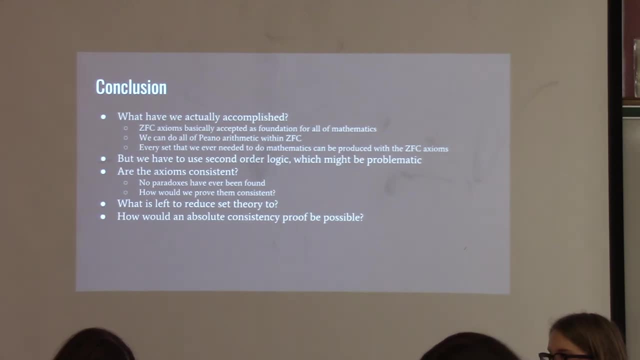 A high-level question, You have to prove it. It's like negative, Negative, Positive, Positive. The other part of the question was this: OK, OK, OK, Wait, Wait. Before anyone answers, just imagine how have we in the past ever shown that something? 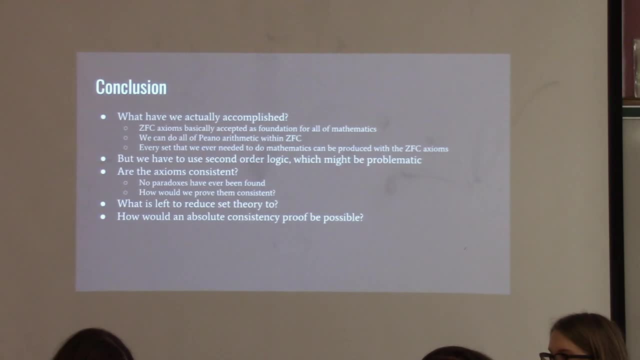 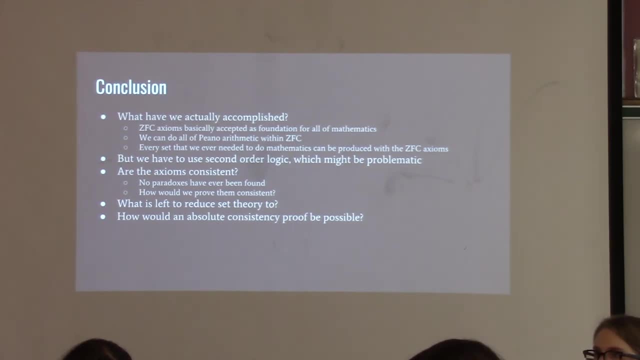 Let's do something lower than ZFC Low. but the very, very bottom is set theory. So if I now have axioms of set theory, because I was forced to axiomatize this branch of mathematics instead of keeping it intuitive because of Russell's paradox, 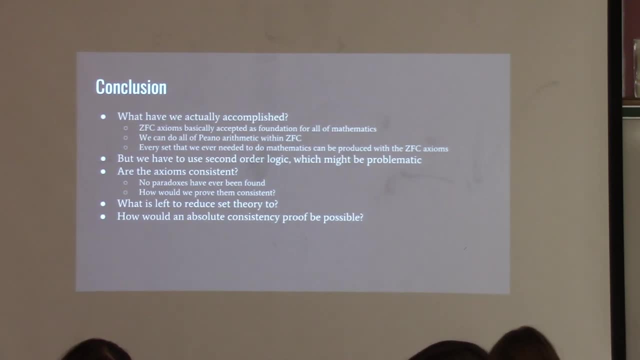 and maybe we would have tried to do that anyway- that now we seem to have run out of mathematical objects. I cannot even imagine what a model of ZFC would look like. It would have to be some kind of even more abstract thing, Something, yeah, pure logic. 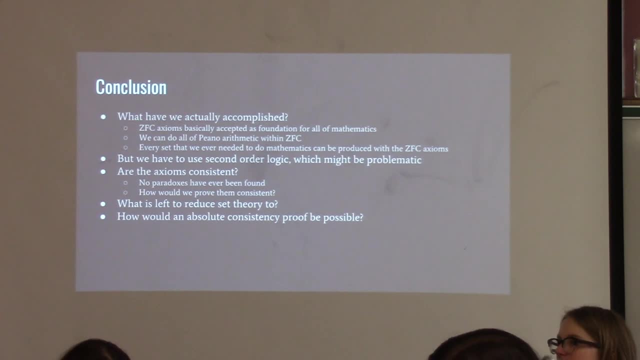 Okay, well, now you're just being Russell, basically right. This is what led him to kind of pursue this, because we've run out, right, Okay. so this is sort of a partial success, at least as of 1925.. 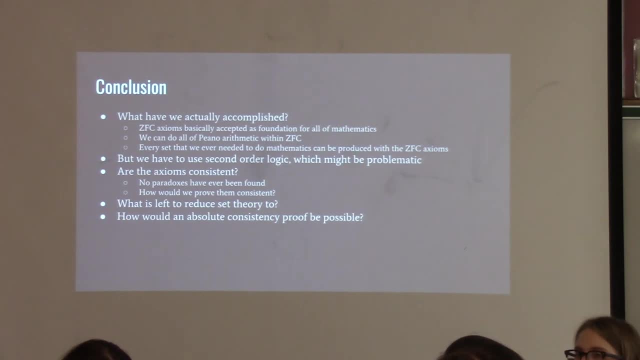 We have an axiomatization of set theory, but we don't know if it's consistent. and until it's consistent we can't truly rest, say some people Wait. and then the other option is like if set theory can demonstrate its own consistency. 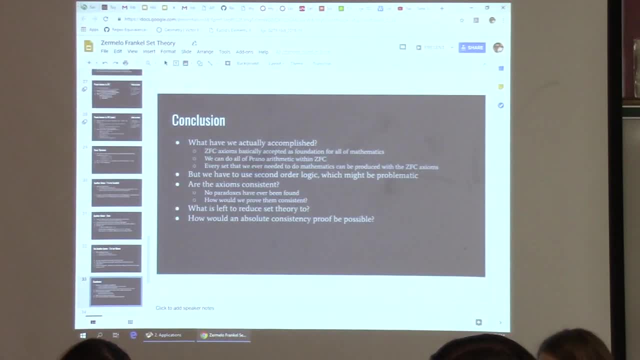 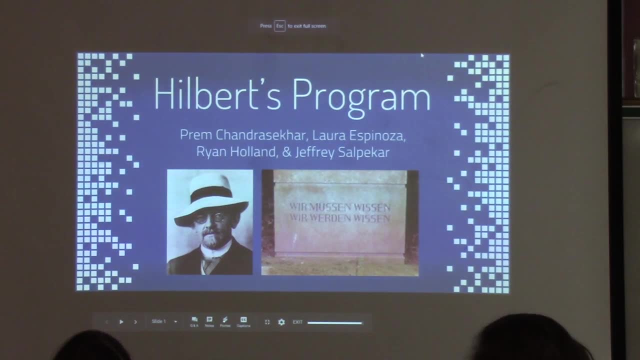 Somehow, whatever that means. Okay, good, All right. so what do we have? A half an hour 35 minutes, All right. good, we can do this. All right, David Hilbert. This is a presentation from last year. 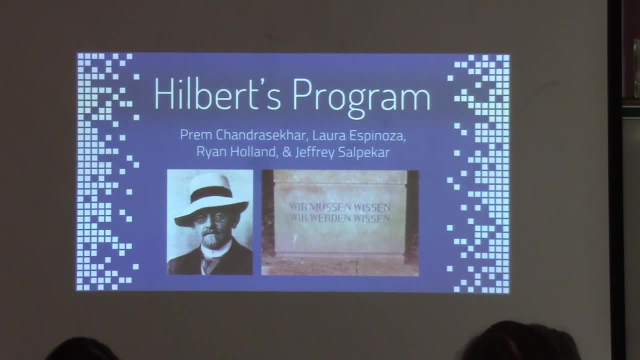 This is David Hilbert. This is such a great picture. He is exactly the guy for this job. He is not going to rest until mathematics has been axiomatized, and axiomatized correctly- and correctly to him means that it has been axiomatized. 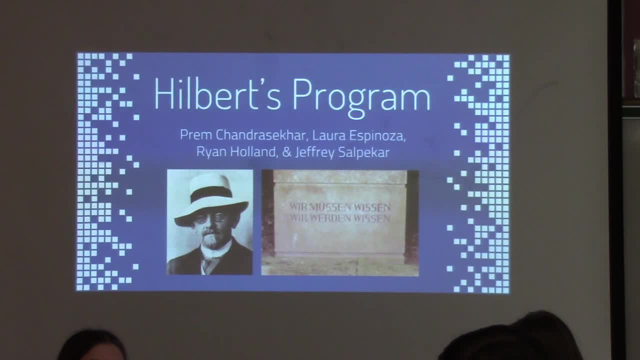 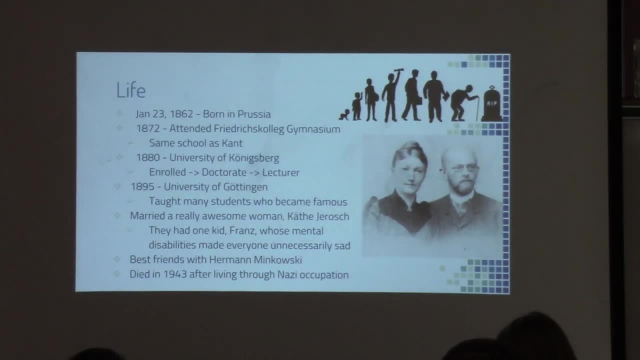 according to these, these metamathematical objectives that he sets for himself, and this is what we're going to review. All right, so what's up with David Hilbert, the person born in Prussia, in German-speaking region of Prussia? 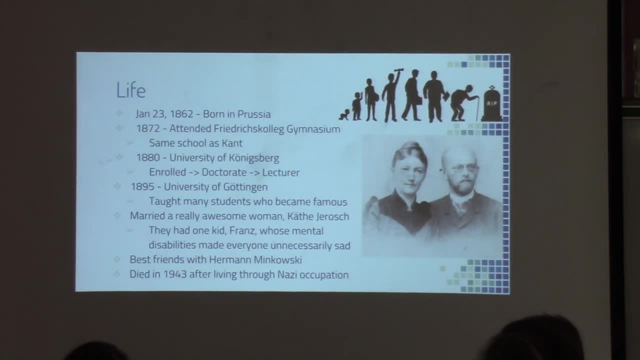 He went to the University of Konigsberg- We may have said all this already. He went to Göttingen. Göttingen becomes basically because of that- because Hilbert is there- the number one university in Germany and Germany is the number one country. 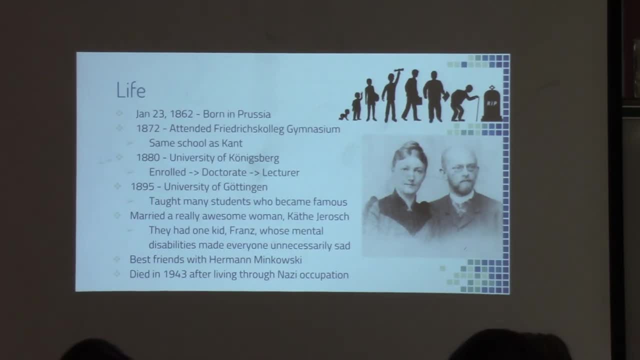 for studying math right Through the 30s or through the mid-30s. He had tons of students who became really famous. The thing about Hilbert is he unlike the intuitionists, unlike Frege- certainly he was like very powerful. 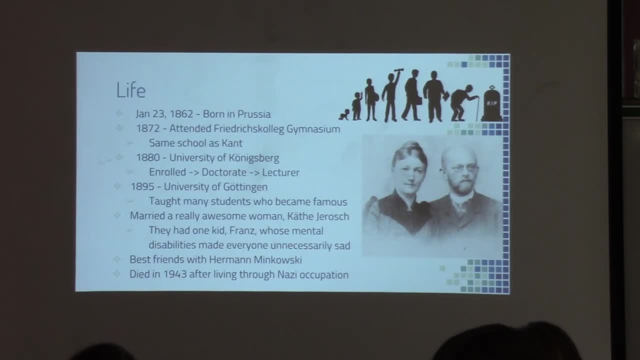 sociologically like powerful or whatever. Like he spoke very forcefully When he did things, people like listened. He like got a lot of people working under them. You know, there's just a whole bunch of people working under him. There's just a whole bunch of people working under him. 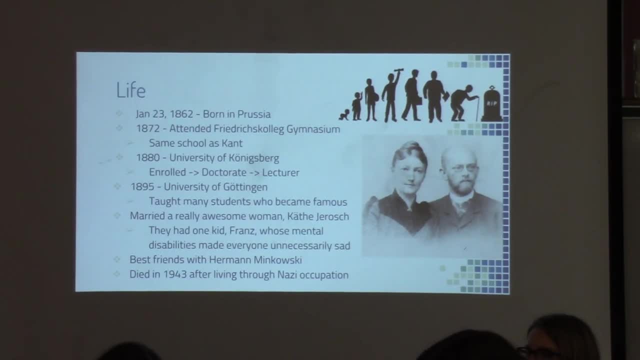 There's a whole team of mathematicians. Basically, he made this whole place where all the top people in the world wanted to go And they all did come And they all came and whatever Hilbert said to do, they did it. 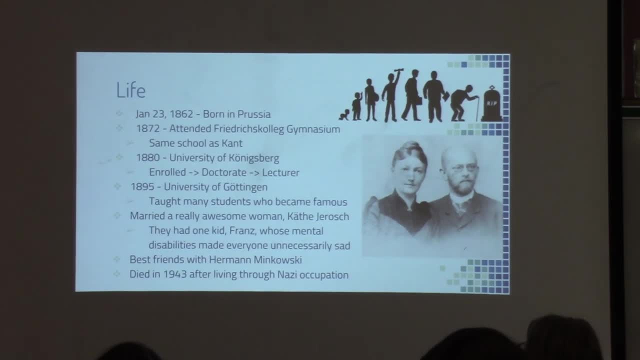 And so his influence on the first third of the 20th century of mathematics was huge. He was not just a guy writing like the perfect script, like home in his house, like you know, screaming at his wife about cookies and stuff. He was like really out there. 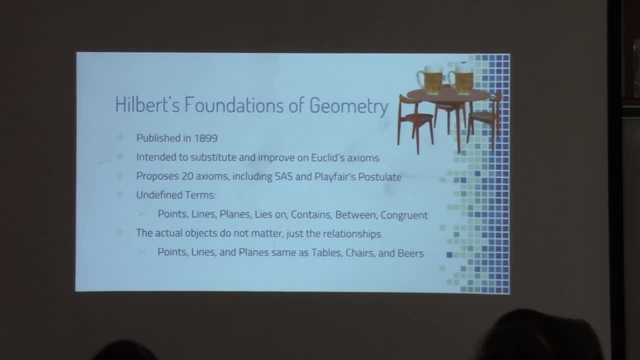 Okay, and we're going to talk about this. Oh, so this is a review. We had a whole other previous presentation: Hilbert's Foundations of Geometry. he published this in 1899. this was like the last, really this was. he takes on this task of. 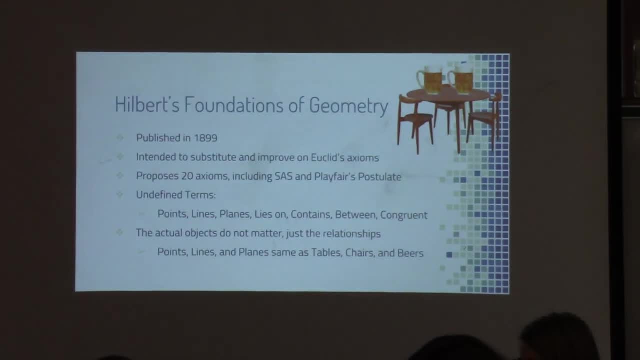 axiomatizing Euclidean geometry. and he basically just does it. and you will recall that he takes a very strong position on undefined terms as being essential for mathematics and in fact we can't define them, we can't even know what they are. the actual objects do not matter, only the relationships matter. 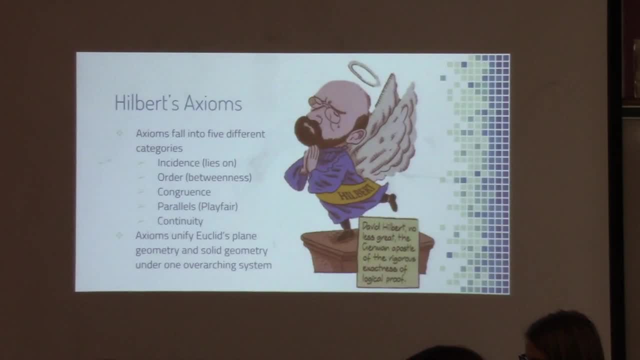 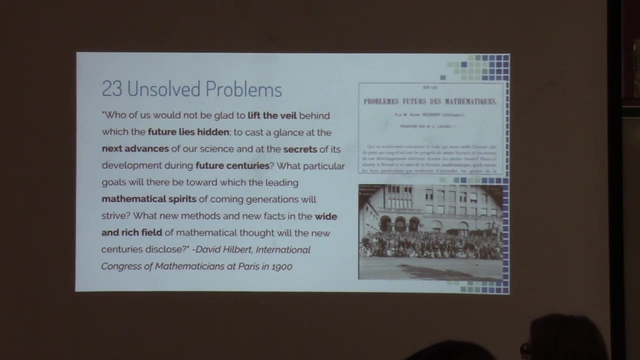 he axiomatizes it and everything is great two years later. I think this is. is it 1900 or 1901? 1900, there is an international congress of mathematicians in Paris in 1900, and everyone is caught up in this sort of feeling of. 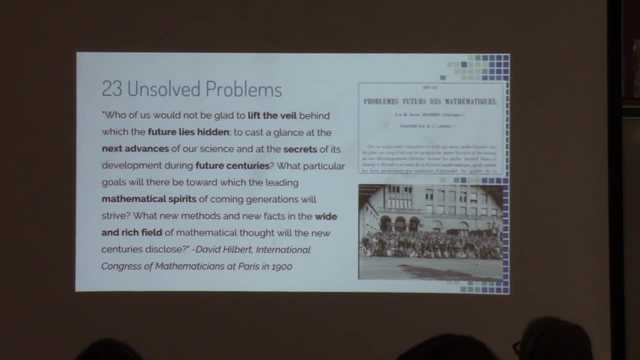 excitement. there's all kinds of new inventions, technology, you know whatever. telephones, steam engine, cool elevators and other exciting things like that are all happening in the pre. what's up, communism, all the things like communism and elevators. 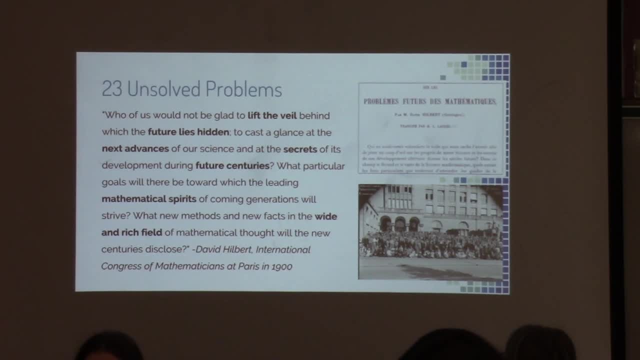 basically the future is now, and so this is a big part of chapter 3 of logic comics. this is toward the end. this is where I stopped reading last class. they all the basically top people in the world all come, and Hilbert got some things to say. 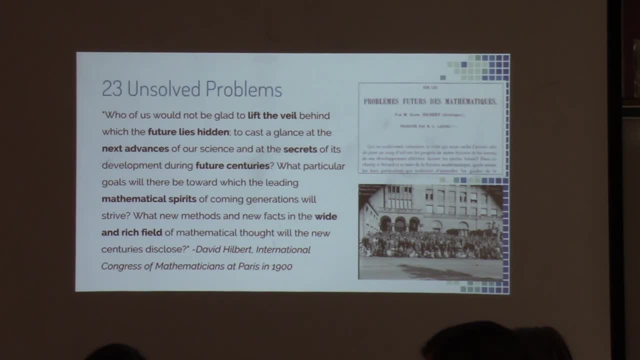 he gives a speech, this famous, famous speech, this speech about the 23 unsolved problems of mathematics. there's a whole backstory which I can't remember exactly the details of. I think they offered him like a slot, as like the headline speaker, or whatever. 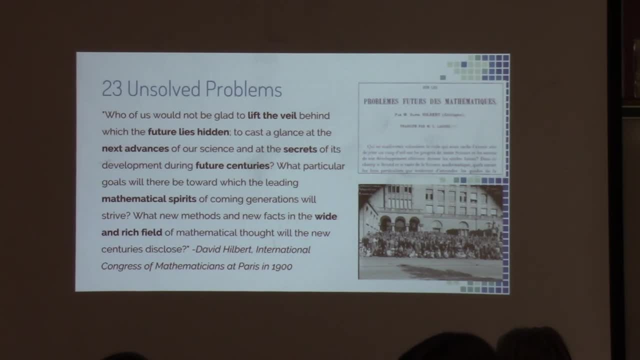 and then he like didn't have his presentation ready in time so he like had to back out and he eventually gave his presentation to like a small room full of like not that many people in like some like in some other weird time slot about something totally unrelated. 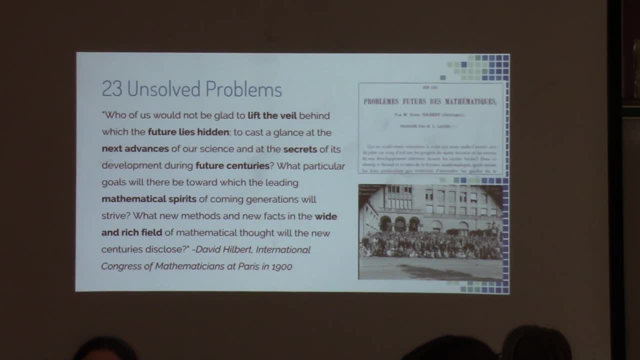 and it only this only became popular like later. so the dramatization in logic comics is not very accurate. in fact, all those people I think like weren't there, like I think Bertrand Russell like wasn't in the room, uh, when this was happening. 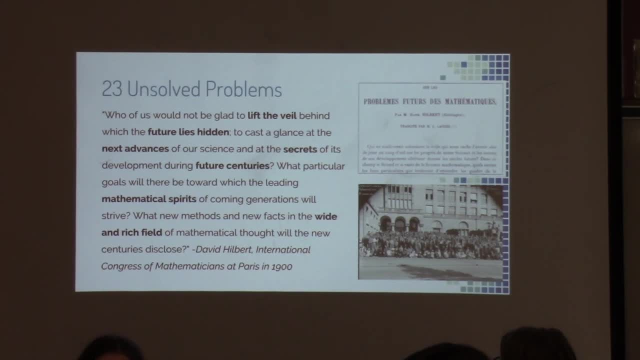 uh, he like left halfway through the conference on like 1-0, uh. but anyway, let's just talk about this stuff and then we'll see you guys in the next one. bye, let's just. let's take the, let's take the, the, the sort of uh, uh, what's it called? very like romantic view of things. 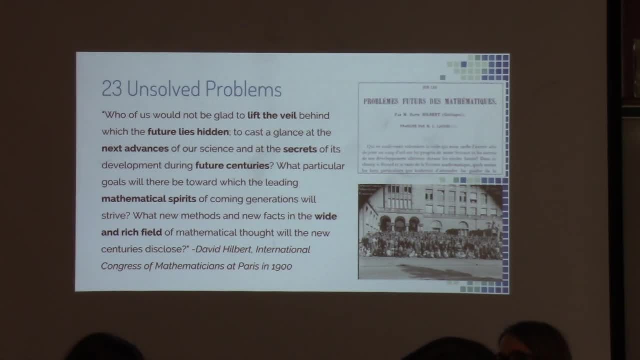 Hilbert comes to Paris and he gives a talk in a grand ballroom with tens of thousands of people and they're all listening and hanging in every word. and he says: who of us would not be glad to lift the veil behind which the future lies hidden? 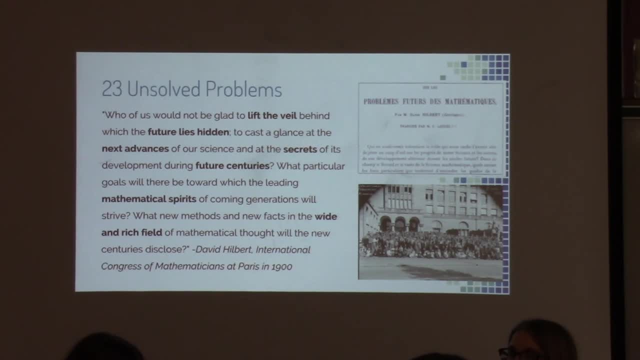 to cast a glance at the next advances of our science and at the secrets of its development during future centuries. what particular goals will there be towards which the leading mathematical spirits of coming generations will strive? what new methods and new facts in the wide and rich field of mathematical thought will the new centuries disclose? 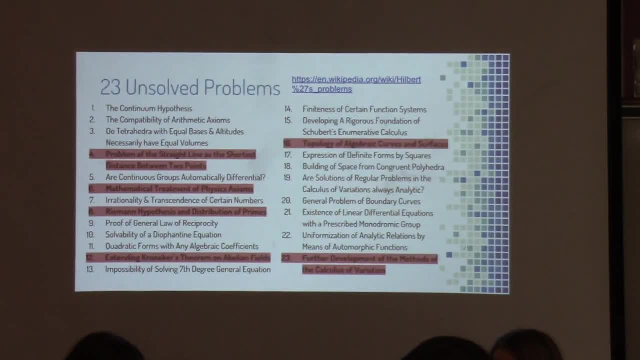 okay. and then he says I got twenty-three problems for you, and what he says is: yo, these are, in my opinion, shut up. I'm David Hilbert, I got this. uh, these are the problems that I feel that should be the most important problems. 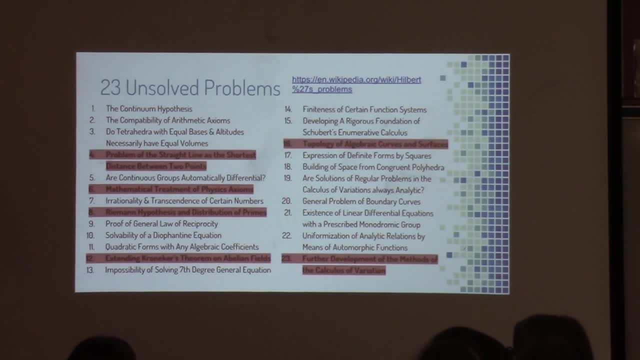 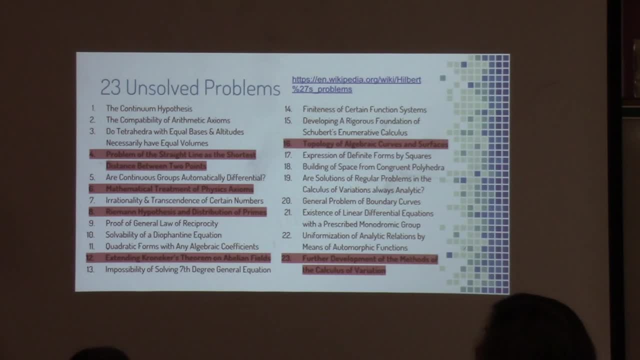 but he was also. this was also a somewhat idiosyncratic list in that he was obsessed with um, the things on the kind of cutting edge of mathematical rigor and mathematical abstraction at that time, and um, in logic comics they do this whole. there's this whole hilarious section in which he, the author of logic comics, sort of envisions the audience as being sort of broken down into the Germans who are all following Weierstrass, obsessed with like rigor, and want all mathematics to be formalized. and then they're like the French mathematicians who are following Poincaré and want to do everything intuitively and think rigor is like sort of silly. this is kind of a caricature, but that's, it is a cartoon after all. 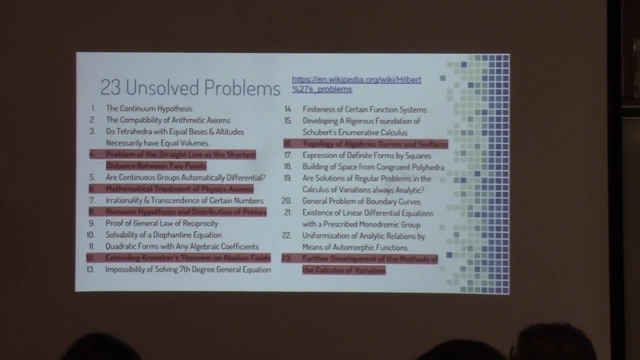 um and uh. I think it's certainly true that not all mathematicians- even in 1900, are following, like the latest you know, explorations into like ordinals and stuff like that. but Hilbert says no, you should. in fact I personally. I think his number one problem, the problem he leads the list off with, is kind of like an FU to anyone who's like not taking Cantor seriously. 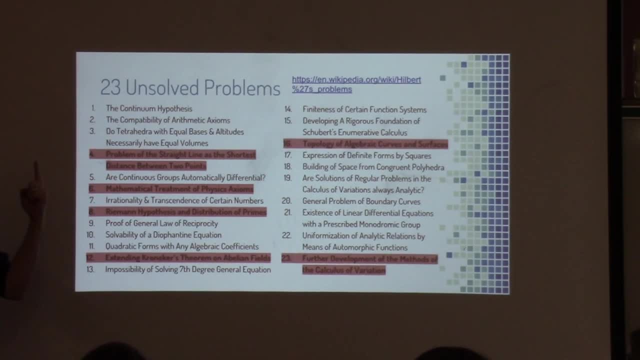 he claims that the very number one problem that should dominate the twentieth century is the Continuum Hypothesis, which is like not a traditional mathematical theory, it's not a theorem at all, it's like this very obscure, you might say abstract, and sort of like, not particularly applicable to like at least, traditional things like physics. 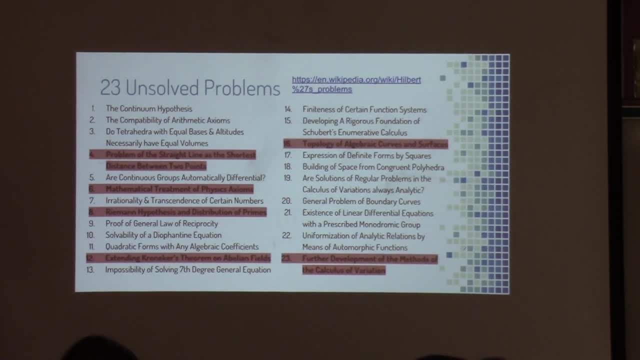 um is there a set whose size is in between that of the natural numbers and the real numbers? um number two: the compatibility of the arithmetic axioms, in other words a proof that the axioms of piano arithmetic are consistent. that's his number two problem. 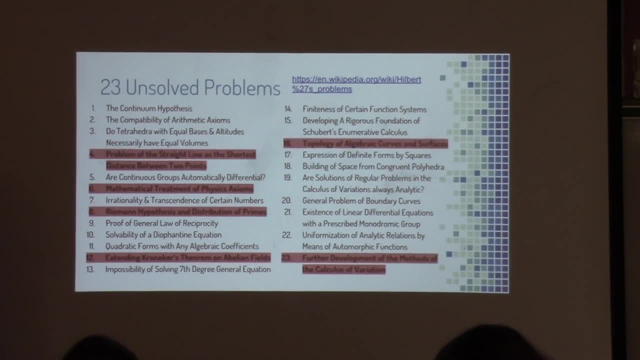 uh, this is pre-Russell's Paradox, by the way. so he's obsessing over consistency in the second of his of his things, something that most other people are not working on. uh, okay, some weird geometry things. uh, the problem of the straight line is the shortest distance between two points. 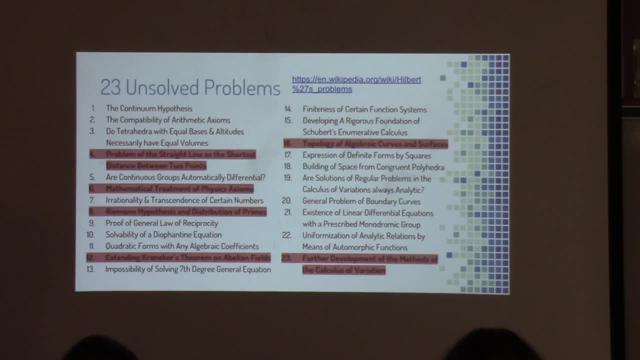 uh, okay, uh, stuff about groups, things that are way over my head. oh hey, by the way, can you just like uh, axiomatize physics. thanks, get back to me when you're done. uh, there are certain numbers which he really wants to know, whether they're transcendental or not. 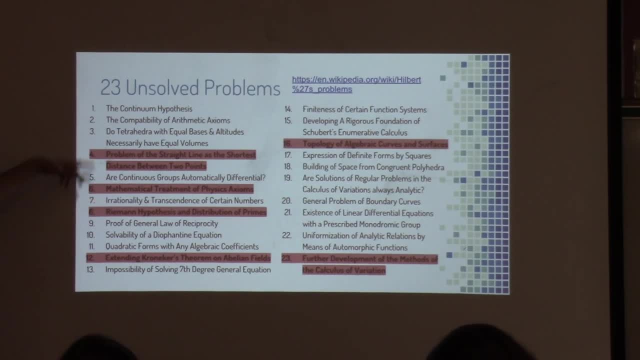 like pi and e and e. I think pi and e were done by then. but like pi to the e, e to the pi, which I mentioned are still not solved. um, the Riemann Hypothesis- okay great, don't know that much about that, so I'm gonna leave that off. 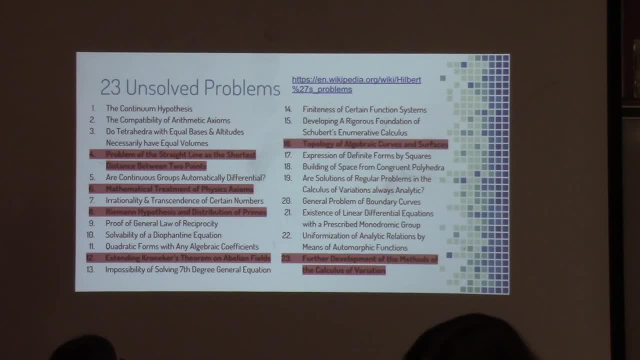 there's a couple slides coming on it, other things um Diophantine Equation. this is kind of relevant to us. what's a Diophantine Equation? has this come up in this class yet? no, no wait. yeah, oh, maybe it did um. 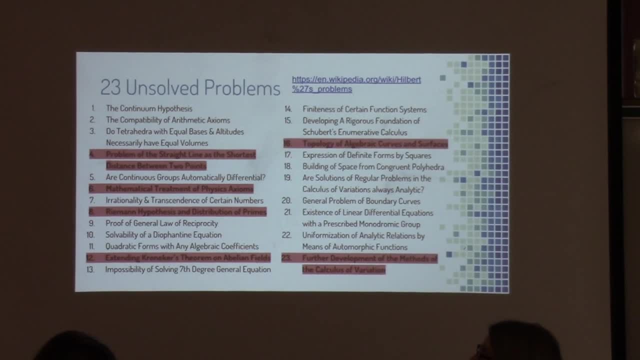 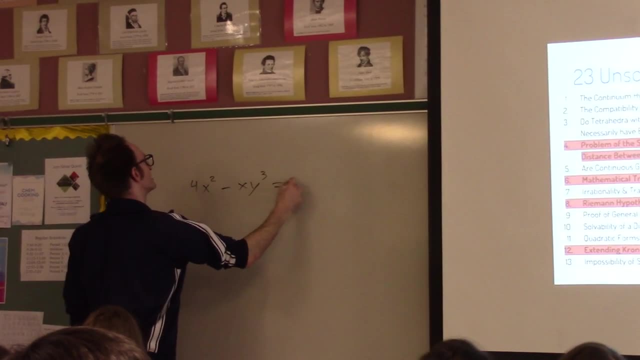 it's a. it's an equation, like of the form. like you know, four x squared- uh, you know, minus xy cubed equals two. we did that's why it's Diophantism. so what's the choice on our first one? 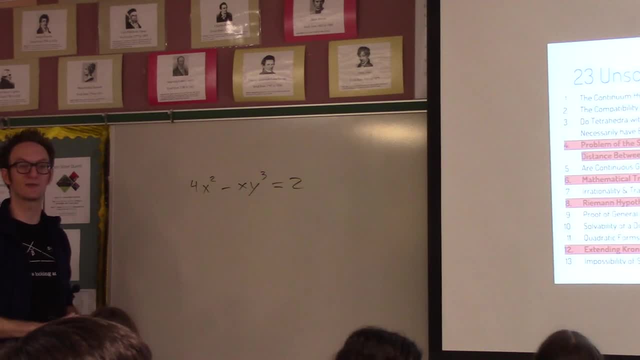 I thought so. I thought it may have. it may have come up extremely briefly anyway, I'll re-mention it now. this is a Diophantine Equation, is an equation which is a polynomial in a certain number of variables and whose only and and. 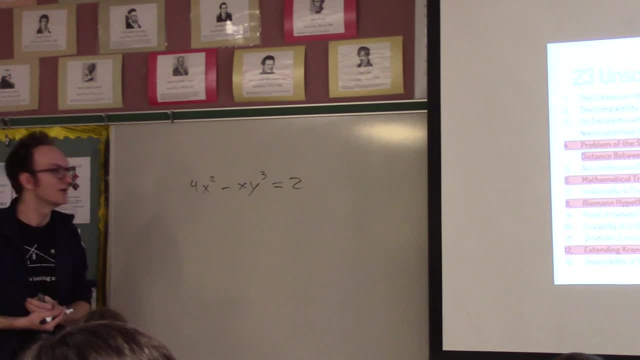 what we seek are solutions which are integers. so do you see any solutions which are integers here? I don't. good, okay, so does. does this equation have integer solutions? I have no idea, um, but is there some general method for solving any Diophantine equation? 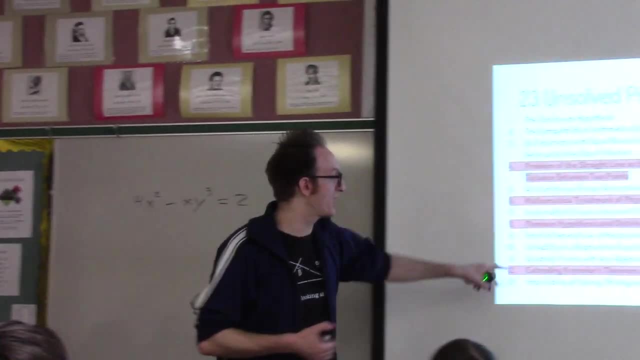 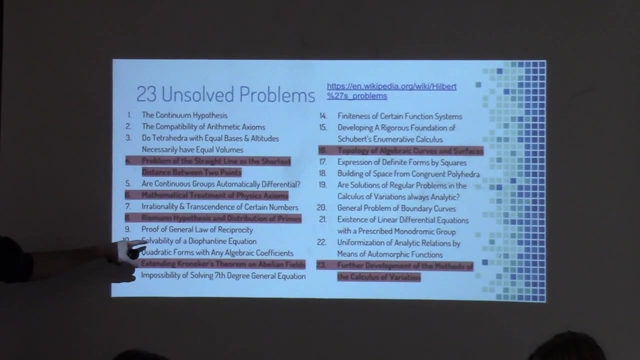 uh, this is what he was looking for. uh, and in fact, what he wants is a algorithm which will tell you for sure whether a given Diophantine equation has solutions and how to find what those solutions are. it seems like there should be one, because, after all, what could be more simple than just like? 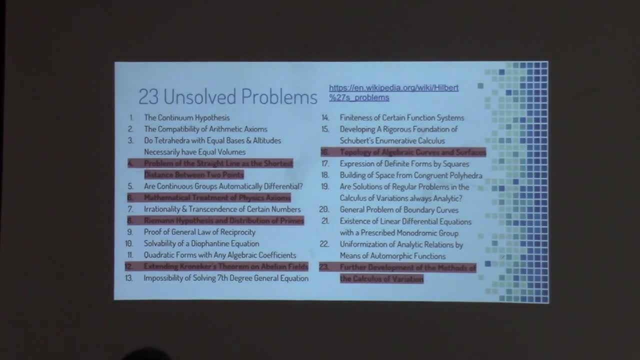 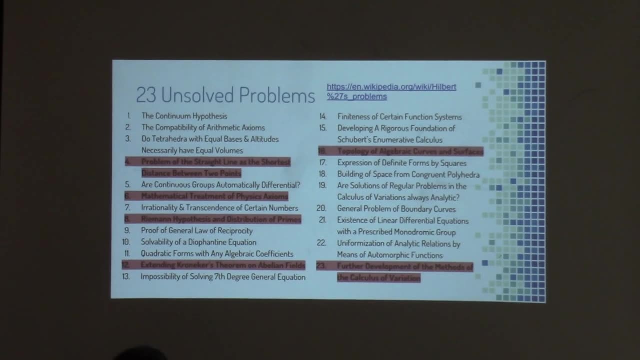 sums and products of like integers, right. so okay, uh, there was none. at that time he thought that was really important. okay, other things, blah, blah. seven degree equation, something, something, something, a lot of stuff is like totally over my head. 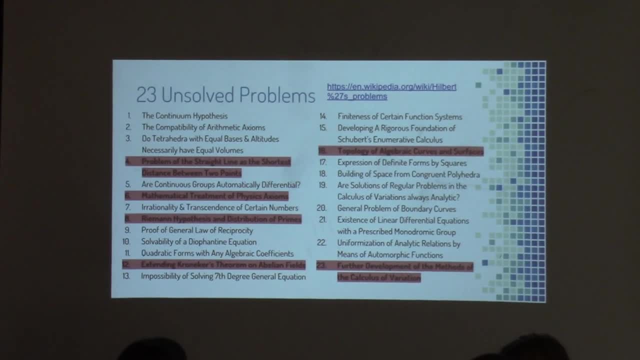 building of space from congruent polyhedra. uh, that sounds exciting. okay, some years we have spent like hours like going through this list one at a time and pulling up the Wikipedia page and like looking at them and stuff. but I don't think I should. we do it anyway for just like one minute. 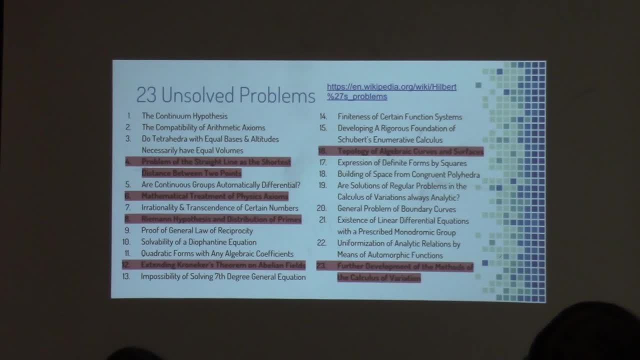 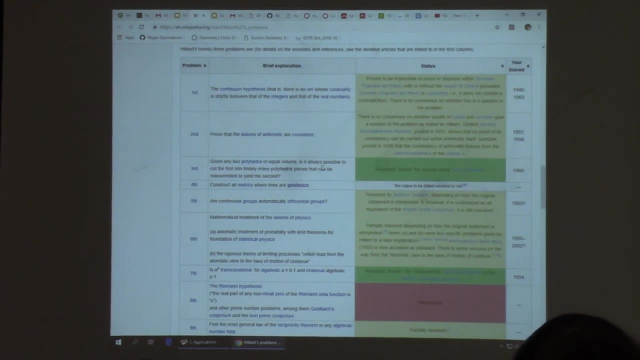 so most of these are either resolvable or partial. ah, what does the color mean? the color green means resolvable. okay, good, so here's the chart and um, what happened is, by and large, people got to work on these problems like right away, and if you solve one of Hilbert's 23 problems, 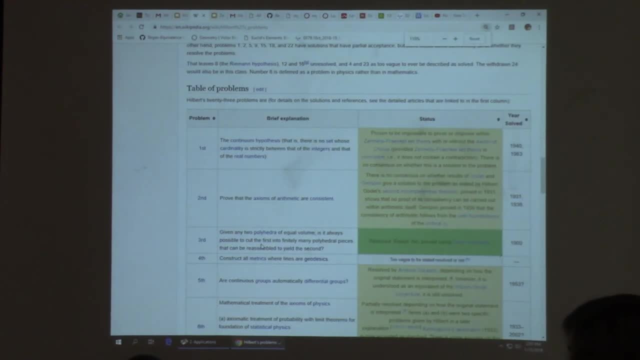 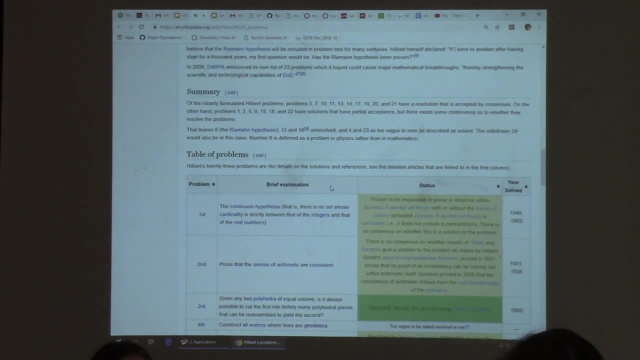 you're just instantly famous and amazing. and here are the problems. and here's this chart. Wikipedia goes through and says, okay, some of this I don't want to talk about because it ruins the idea that there's more things coming. but first problem: continuum hypothesis. 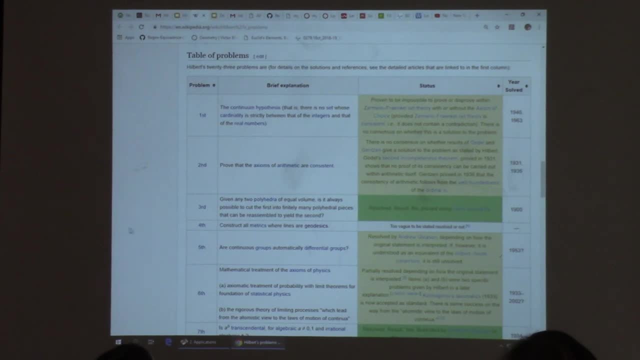 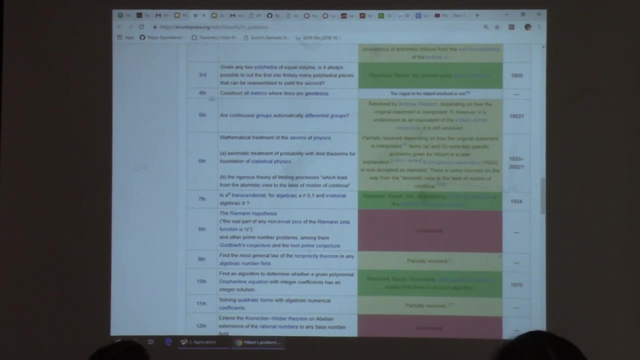 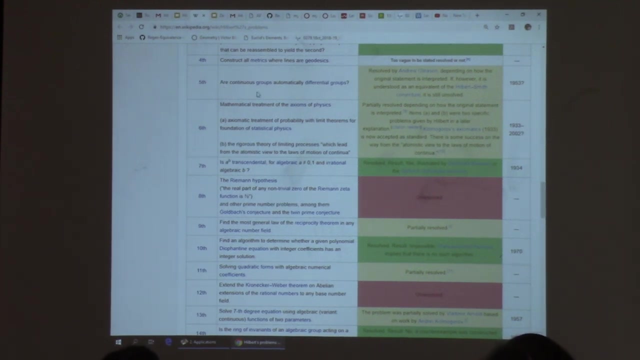 uh sorry. second problem: uh, third problem resolved. answer: no good. um then fourth problem: uh, too vague to be determined, sorry, Hilbert, please do better. um continuous groups, something, something resolved, ish. um axiomatized physics- partially resolved, okay, um. 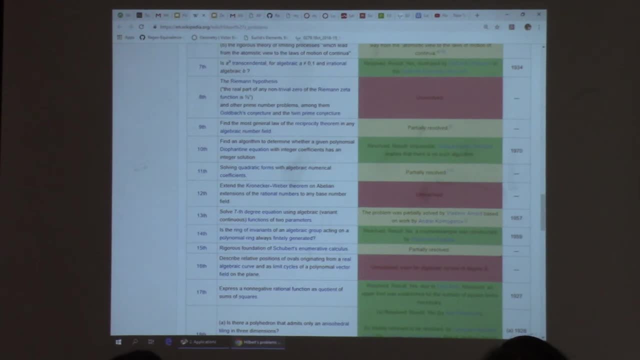 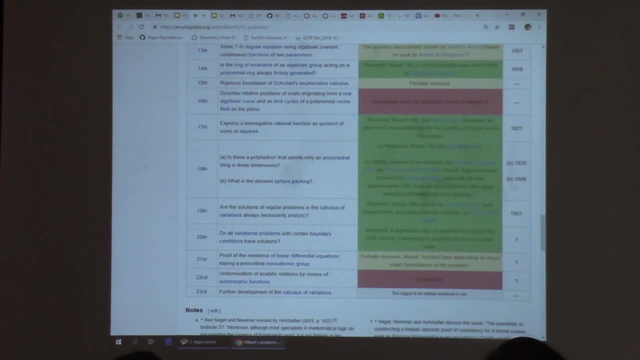 then, is A to the B transcendental, resolved, yes, uh good. the Riemann hypothesis unresolved, um and then, et cetera, et cetera. so, as you can see, like I don't know, about a third of them have been solved. some have been declared too vague to be solved. 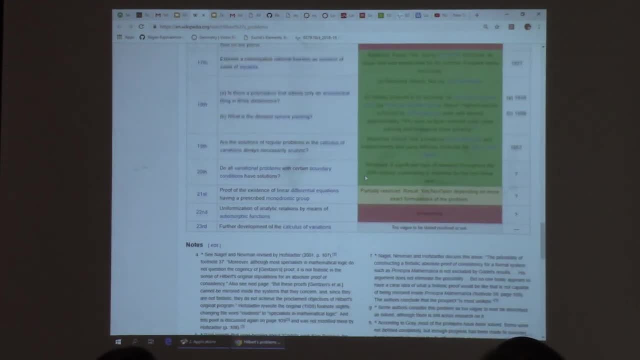 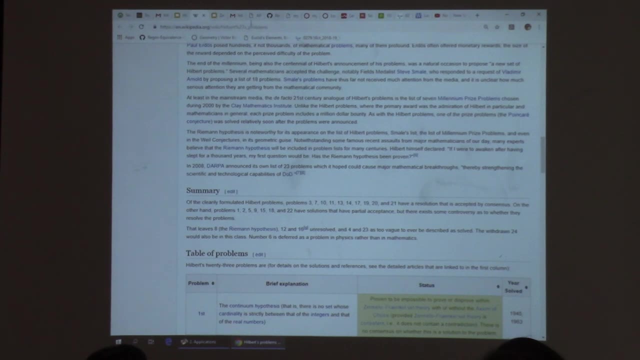 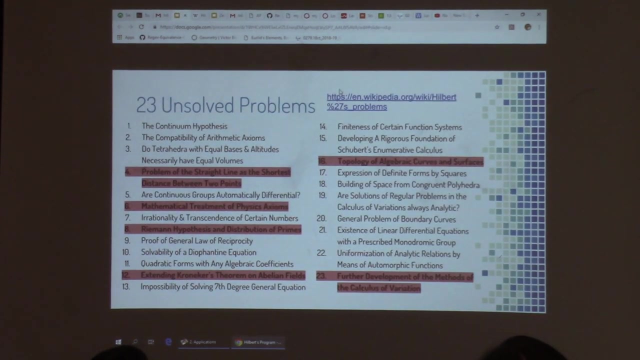 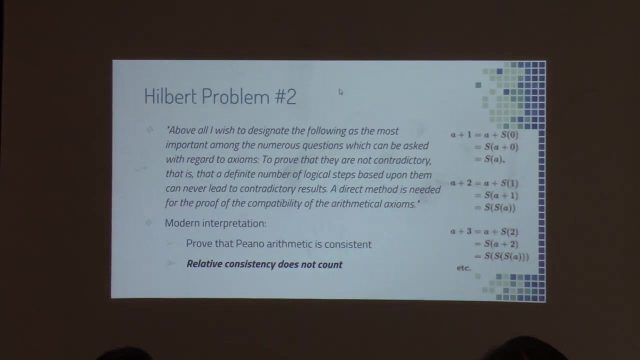 some are still just unresolved. um and uh- yeah, I mean this really- uh, uh, in particular Hilbert problem number two. this is a quote from his paper. above all, I wish to designate the following as the most important among the numerous questions which can be asked in regards to axioms: 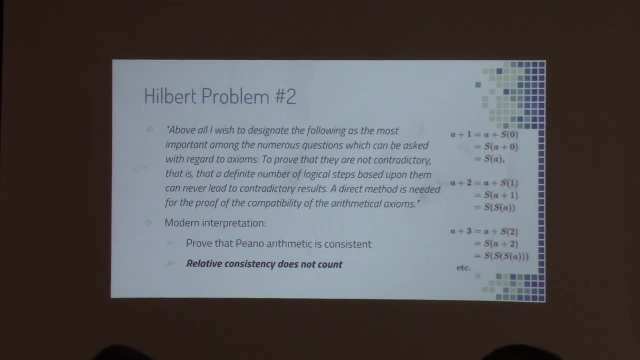 to prove that they are not contradictory, that is, that a definite number of logical steps based upon them can never lead to contradictory results. a direct method is needed for the proof of the compatibility of the arithmetical axioms. this is Hilbert in 1900. 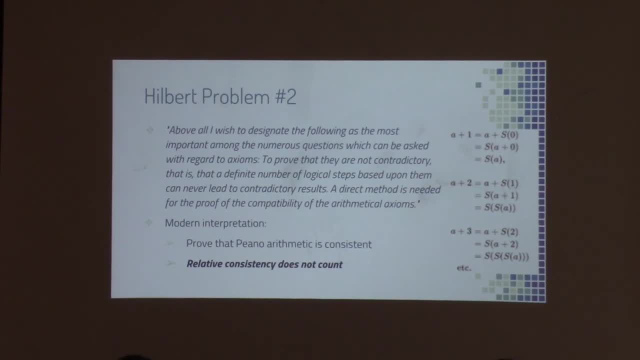 obsessing over the consistency of the axioms of piano arithmetic when almost no other working mathematician is really obsessing over this? do you see how he has placed metamathematics in its primary role? in mathematics, his first two problems are the continuum hypothesis about the existence. 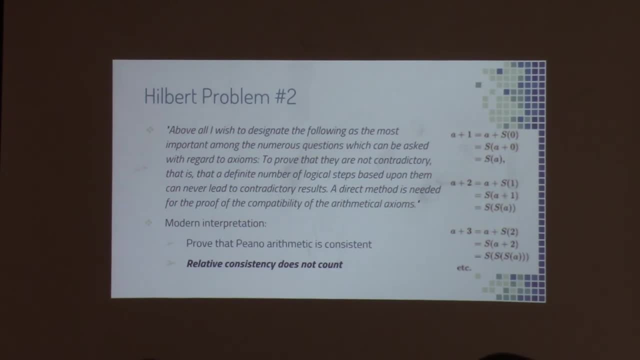 of sets of infinite size and basically showing this is effectively a metamathematical result that he wants. this is before russell's paradox. do you see how, like after russell's paradox, people might have suddenly turned to hilbert as, like the savior, he was the one guy out there? 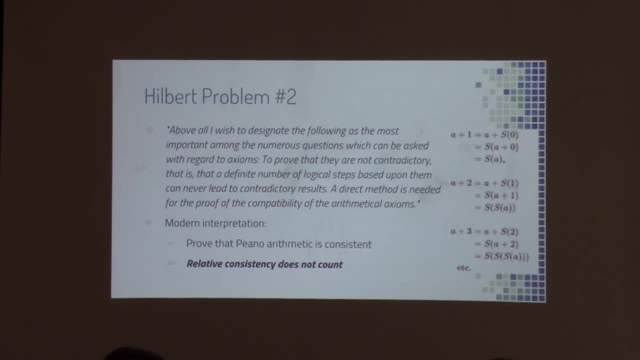 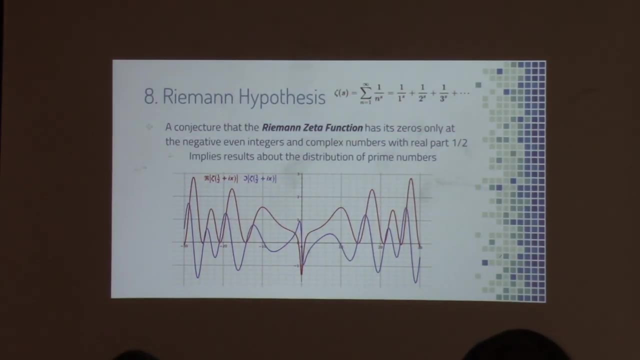 he's not the only guy, but he was the main guy who was obsessing over the need to prove your axioms consistent. okay, the Riemann hypothesis. we could spend one minute talking about this, or an hour. um, conveniently, we only have one minute, because i don't really understand this. 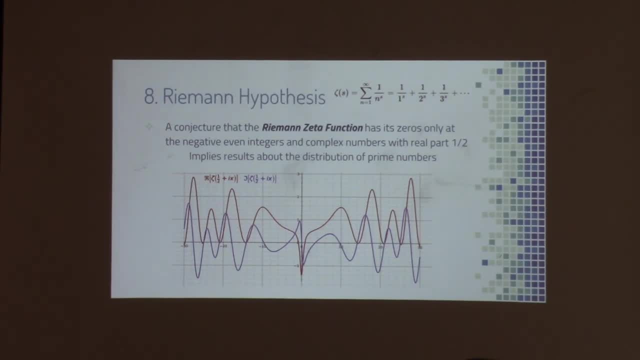 um, oftentimes i've just yielded the floor to like stave or whatever to like just talk about it like this, but we don't really have any time. it's really important. um, it has to do with the distribution of prime numbers. it's- it's phrased as a fact- about complex numbers. 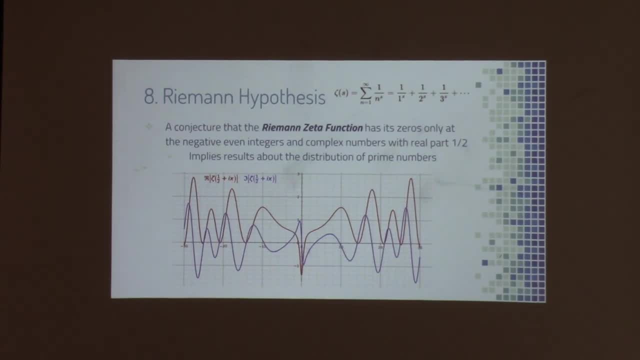 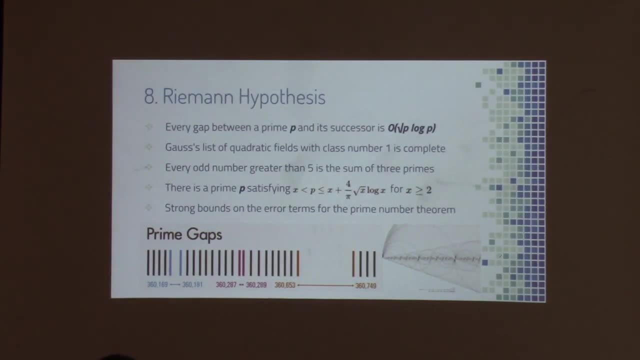 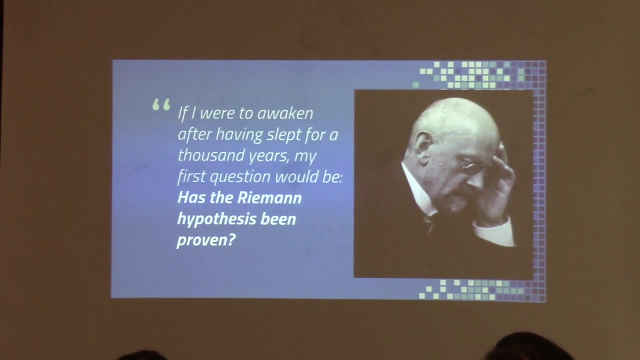 um, see some people who think they know things. uh, if you want more information about this, there are also some great videos on youtube about it. and also, uh, blah, blah, blah, blah. hilbert says: if i were to awaken after having slept for a thousand years, my first question: before i'm like 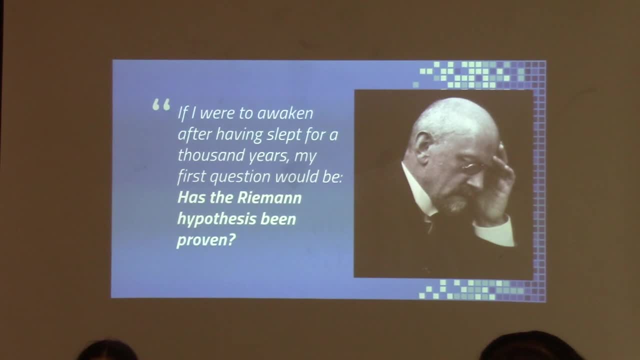 has the Riemann hypothesis come true? no, has the Riemann hypothesis been proven? and the answer is no, it has not been proven and it is. it is still generally considered the most important unproved. unproved sort of conjecture in mathematics. important in the sense that 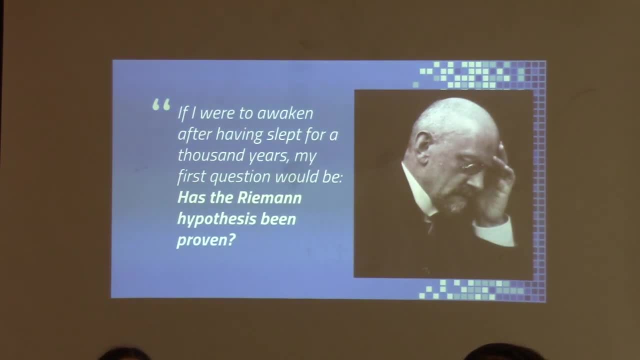 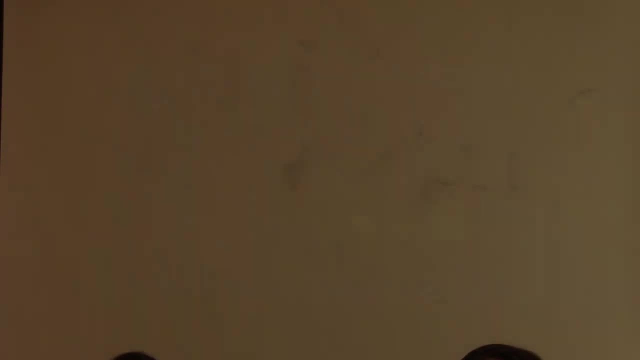 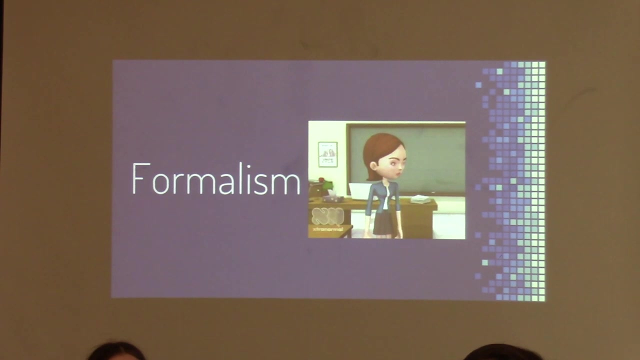 if it's true, then many it has. it has ramifications in like many, many different branches of mathematics at like a somewhat deep level. but this is all. i'm not the authority on this at all, okay, so, uh, what good? uh, remember this video on the rigger day. 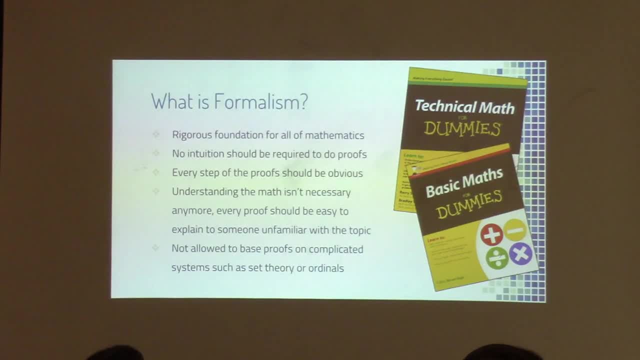 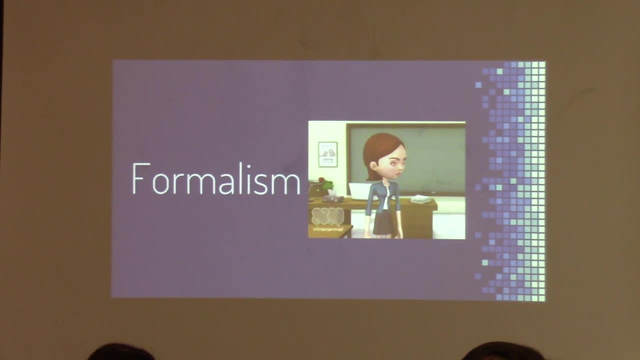 yeah, uh, good, um, all right. so hilbert establishes something which is, which is eventually referred to as hilbert's program, and hilbert's program is: hey, all the top mathematicians in the world, come to gonagin and we're gonna fix everything, all right? 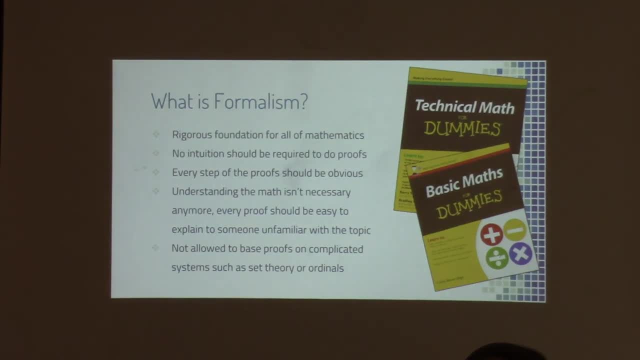 what are we gonna do in gonagin hilbert? well, first of all, um, you can get in the door. you have to sign my contract that says you are a formalist. and what is a formalist? it is hilbert's philosophy of metamathematics. 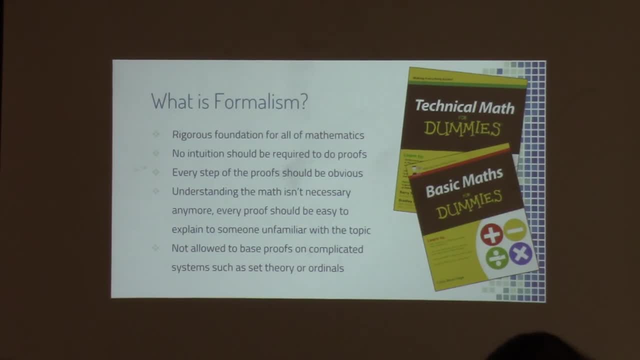 which we discussed, i think, uh pretty well, uh like two weeks ago. but let's say it again, and we are. this is a little bit of a caricature. it's unclear whether hilbert really believes this is kind of a straw man to some extent, but formalism is. 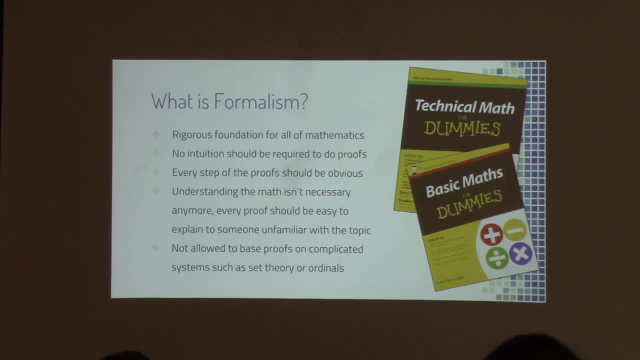 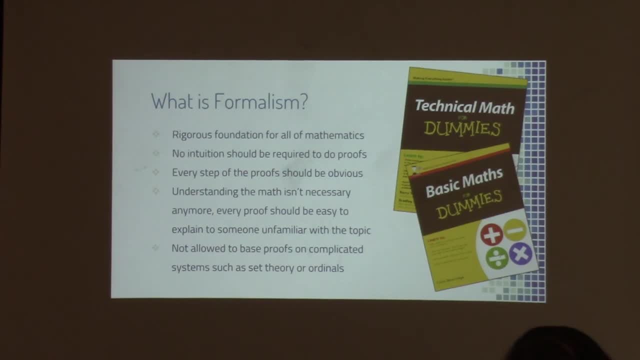 every step of the proof should be an obvious consequence from the previous one, and we shouldn't even have to understand the math anymore. every proof should be easy to explain to someone, even if they don't know anything about the topic, just by going through the logic and 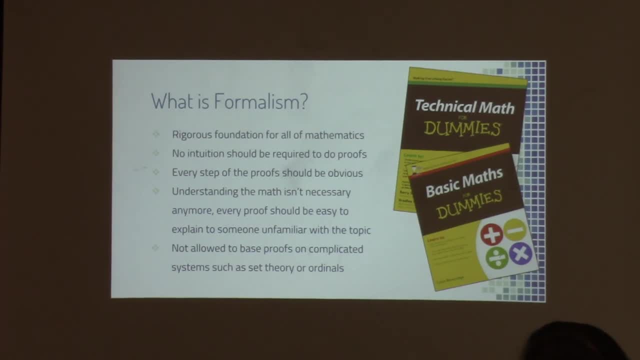 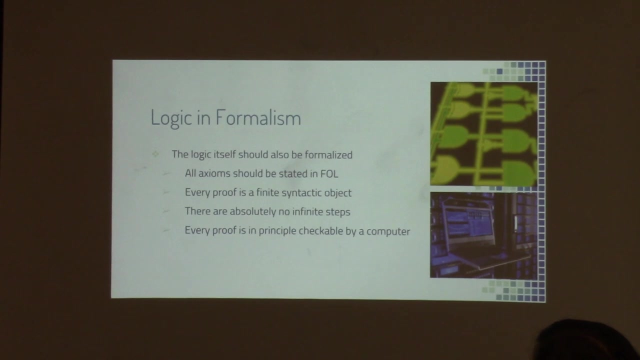 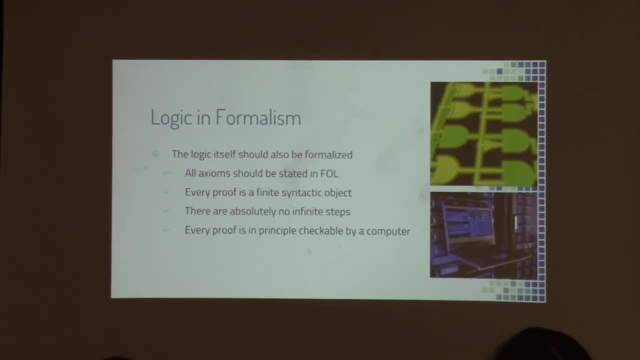 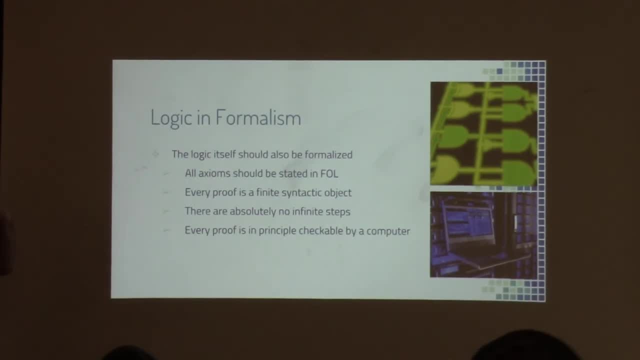 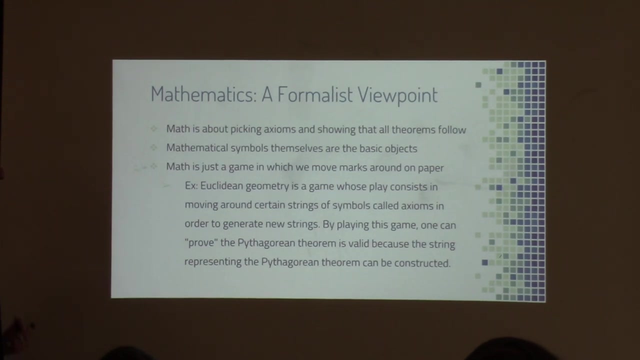 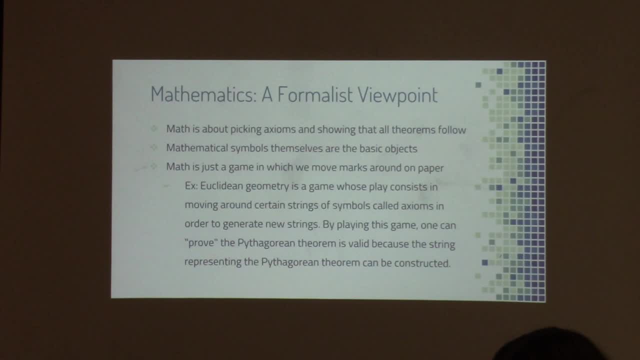 and so we never really know even what the objects of mathematics are. you might even say that the objects of mathematics are the symbols themselves, or something like that, And according to this formalist view, this is a bit of a caricature of the formalist view. 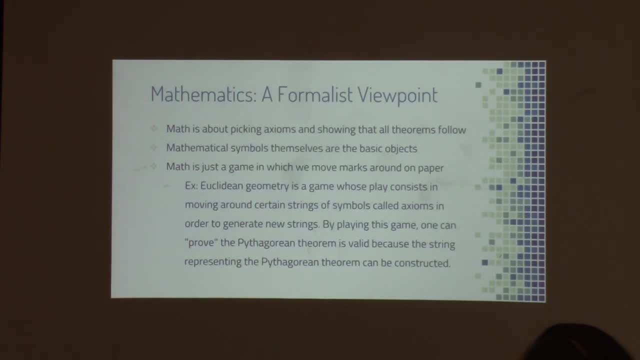 but they do kind of believe this, some of them. Math is just like this game in which we are moving sort of marks around on a piece of paper. This is the end result now of our sort of centuries of rigor, And math now is just Euclidean geometry, for example. 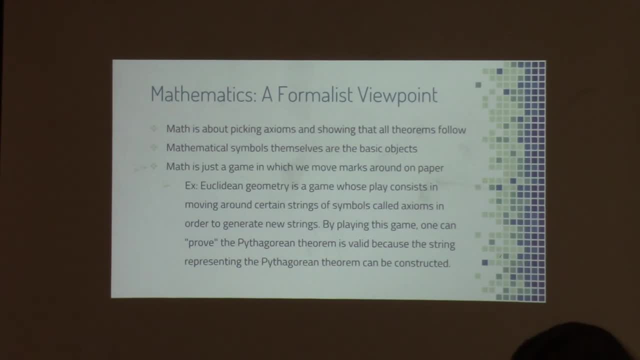 It's a game. You give me some axioms and I use these axioms, which are just strings, and I play this game called Fitch-style proofs, and what that game does is it produces new strings, and that's called doing geometry. 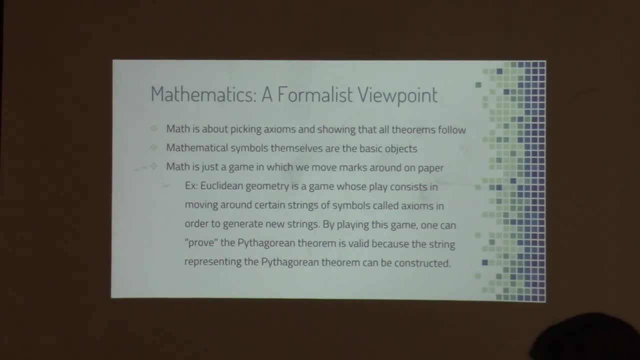 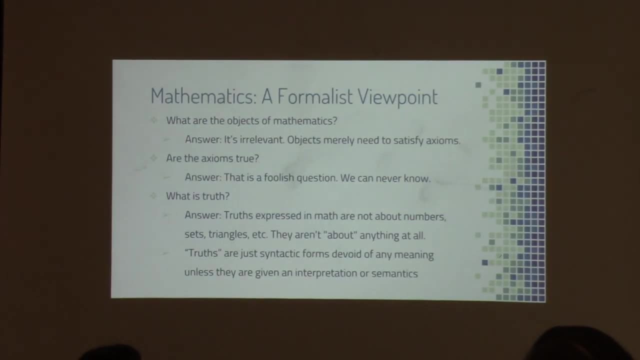 If you're an ultra-formalist, that's what you believe mathematics is. Mathematics is a game of cranking out. It's a game of cranking out theorems based on other theorems. okay, And what are the objects of mathematics to a formalist? 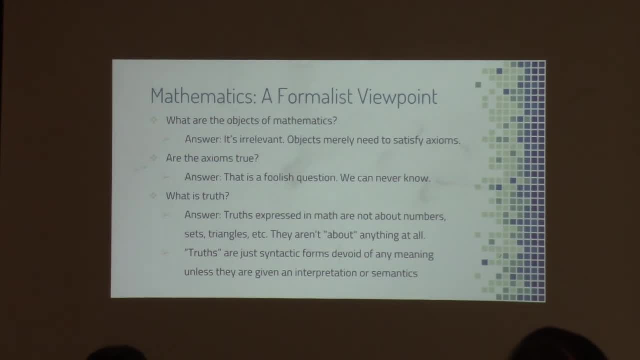 It is irrelevant. You cannot ask that question, and if you do ask it, I refuse to answer it. Objects must merely satisfy axioms, and any object which satisfies the axioms works just as well. So we never really know what objects we're talking about. 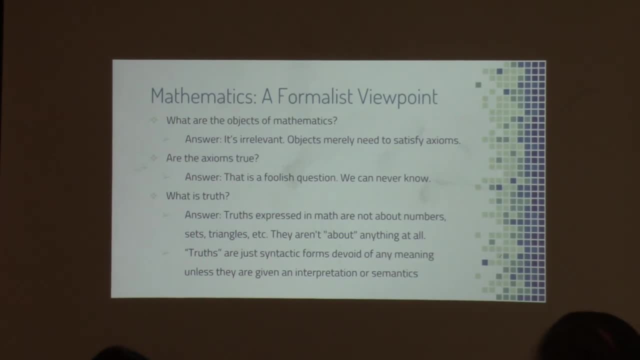 Are the axioms true? Again, Hilbert would say foolish question. You cannot ask that question. I will not answer it. All we can do is come up with our axioms and you could think they're true, but there's no way to prove they're true. 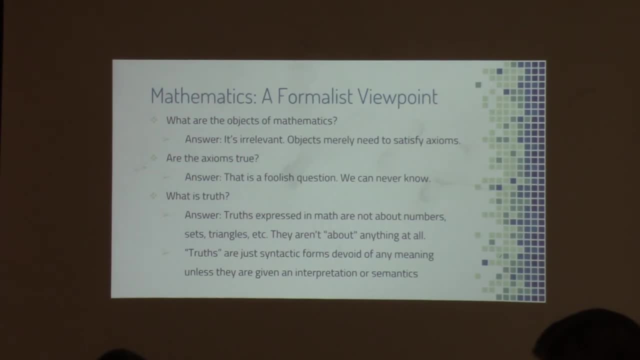 Okay, and what is even truth? I don't even know. right, We don't have truth anymore. All we have are axioms and theorems, and if you prefer to think of the axioms as being true, you can. 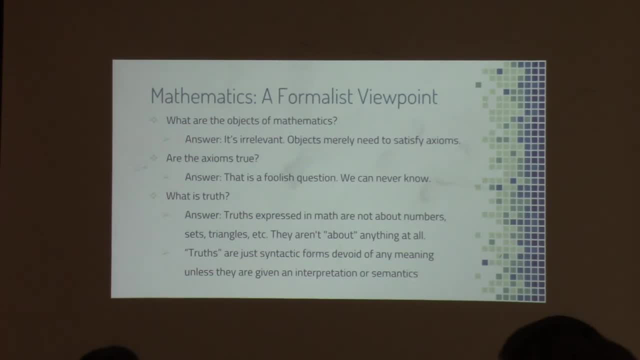 but I can't argue to you that those axioms are true, because I don't even know what objects there are that I'm talking about with these axioms. Anyway, it's kind of a little bit crazy, do you agree? This is like where rigor takes you if you go all the way. 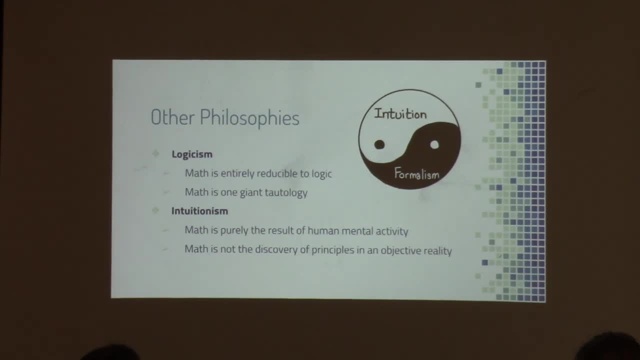 All right, and just to contrast this with the other philosophies of mathematics, there is the logicist philosophy of mathematics. What's up? I think the y dot shouldn't be there Because There's no intuition. Yeah, I think we could just get rid of that yin-yang entirely.